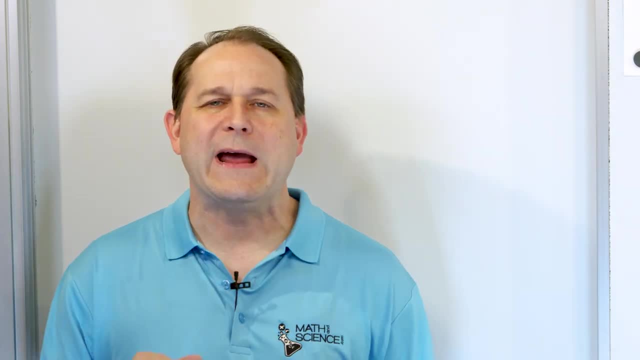 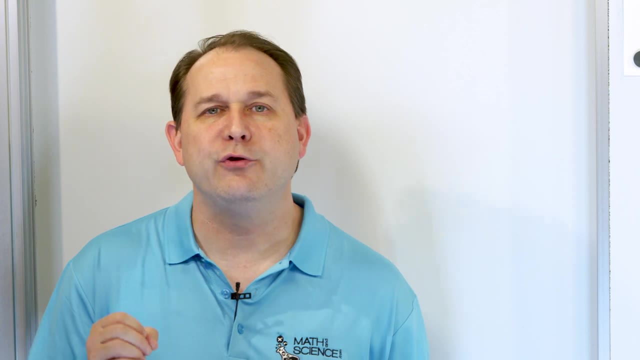 you'll know exactly how it was done, because we're going to do it together. Once we have the frequency table in place, we'll be able to answer some questions about the data. Now, a frequency table is a very common way to present what we call statistical data, And you have lots and lots and. 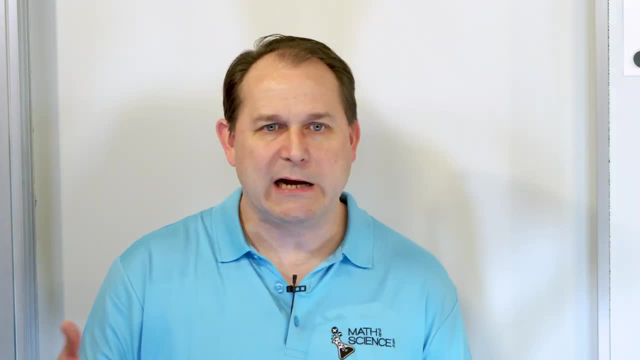 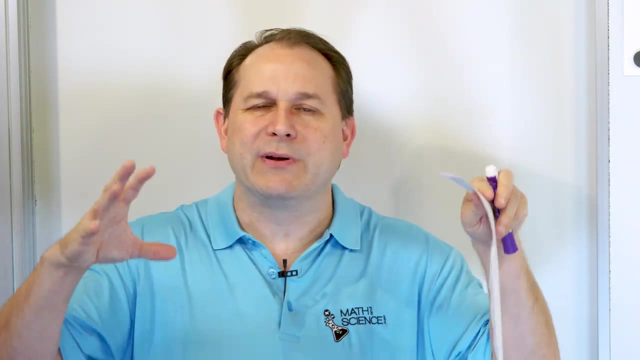 lots of numbers. You know, if I give you 500 numbers and just put them in a line, I mean nobody's going to be able to do anything with that. A frequency table is a really good way to sort of represent all of the data in one place in an easy to digest format. All right, 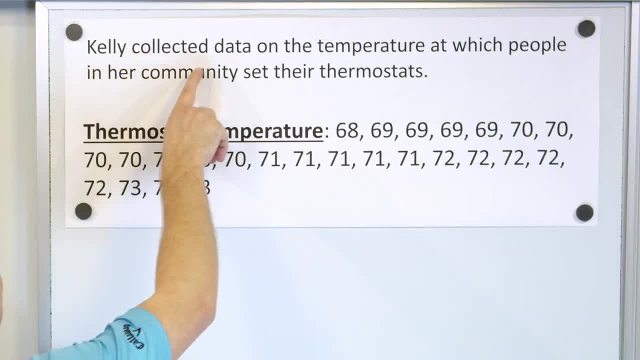 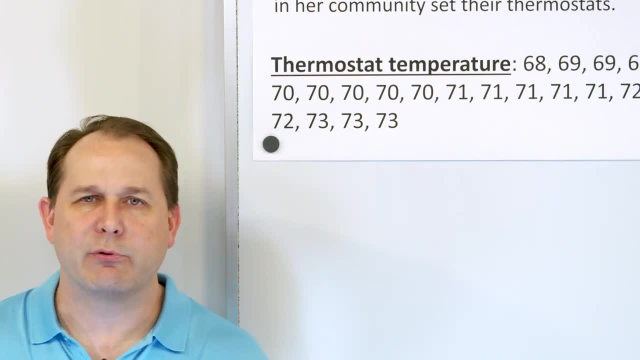 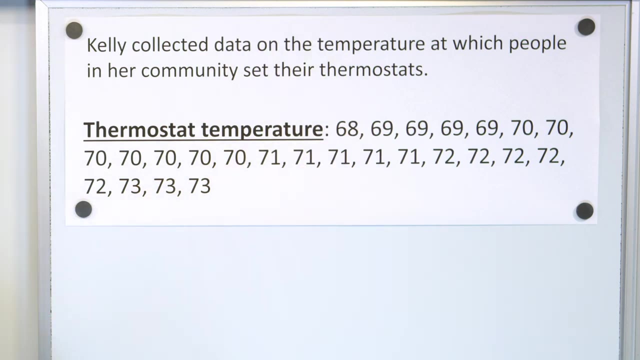 So for our first problem we say: Kelly collected data on the temperature at which people in her community set their thermostats. So basically, houses in the neighborhood. she goes down the street and says: what temperature do you like to set your thermostat at? One person says 68 degrees. She 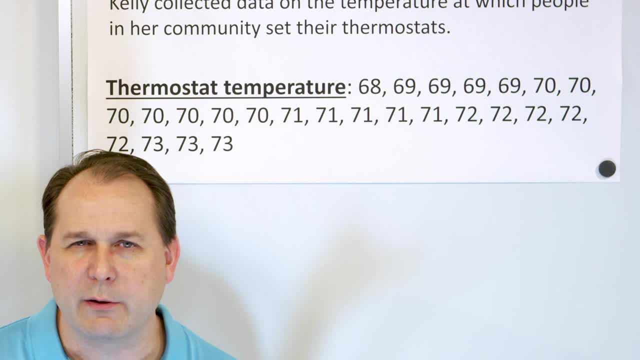 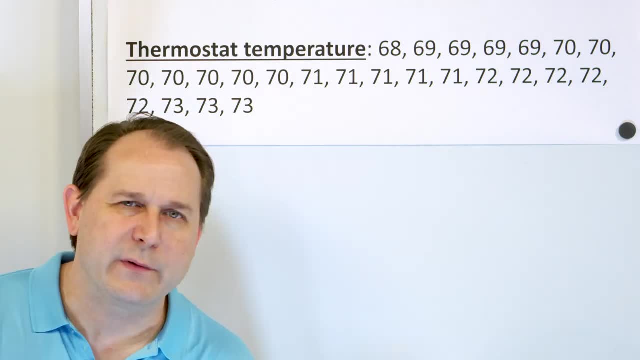 goes next door, that person says 69 degrees, and so on. I have all the numbers here Now. I've already put them in order. In reality, it'll be very random. One person will say 80 degrees, next person will say 73 degrees. These are all in Fahrenheit, but you know. 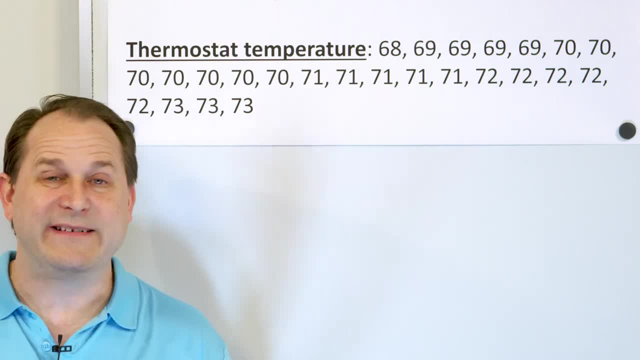 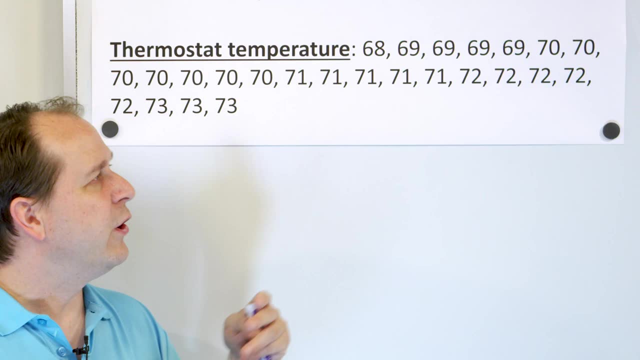 it doesn't the point, it doesn't matter. The temperature scale we're in could be Celsius, could be Kelvin, which is another temperature scale we'll learn about later in chemistry and in physics. These are in Fahrenheit. Okay, So we have all of the data here and I've already put it in order of. 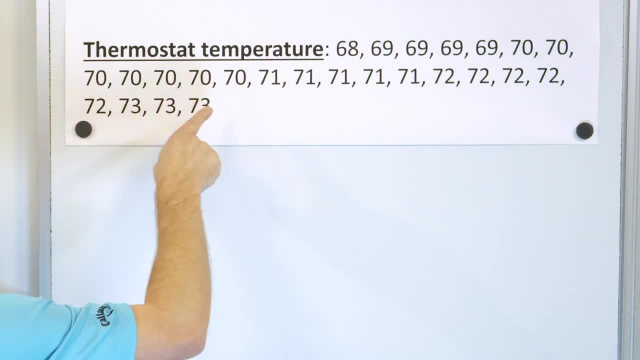 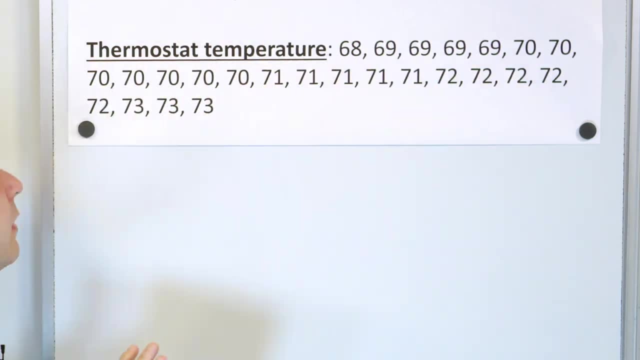 least to greatest. So every number you see here is a different house. So you can see lots of people chose to put their temperature at 70 degrees, Lots of people chose 71,, lots of people chose 72 and so on. But still look at all those numbers. If you look at all the numbers and just try to understand. 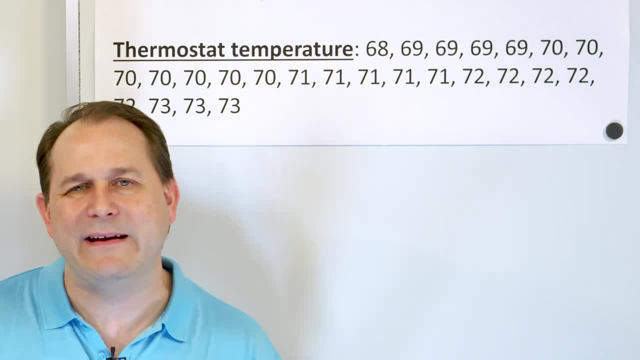 what everyone in the neighborhood is doing. just by looking at the numbers you can see that the temperature is going up. So if you look at all the numbers and just try to understand what everyone in the neighborhood is doing just by looking at numbers, it's basically impossible, because you have all these numbers and we're not. 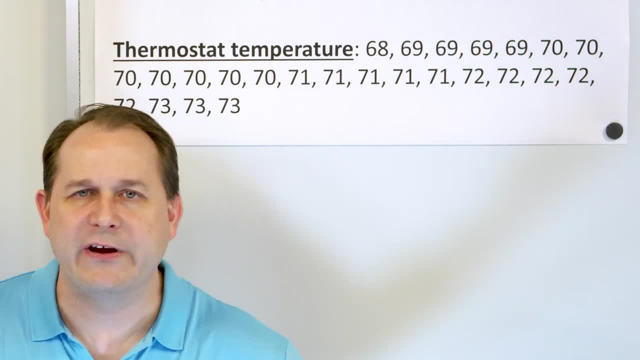 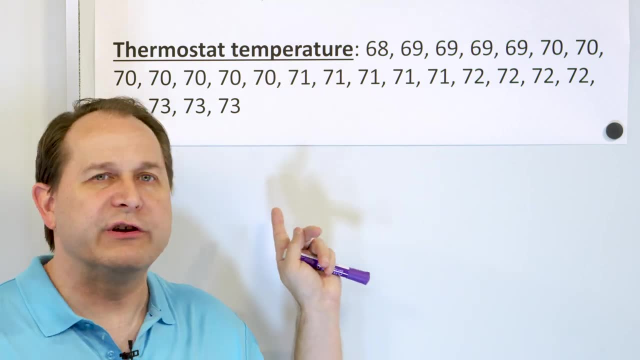 human computers, And so I can't really tell you how many percent of people prefer to have their temperature above 73 degrees, For instance. I can't easily see that. So what we're going to do is construct a table to summarize this information, And it's called a frequency table, The word 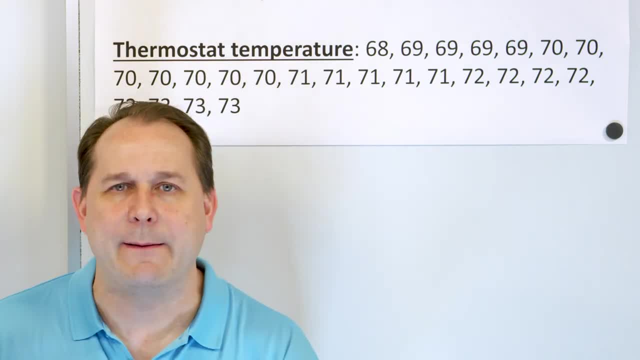 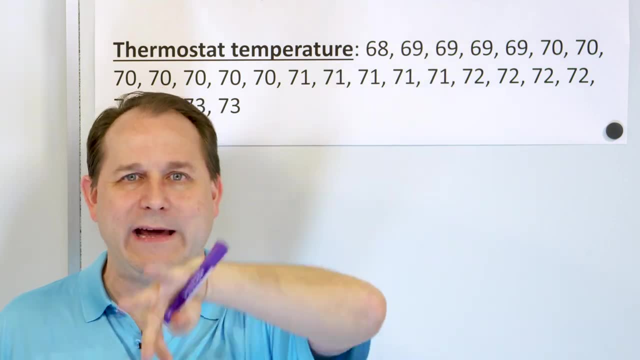 frequency. um. frequency means how frequent something is happening. There's a science definition. We'll talk about frequency of waves. We'll talk about that later. Higher frequency is a faster wiggling wave right, The faster it goes up and down. But in this context, when we say the 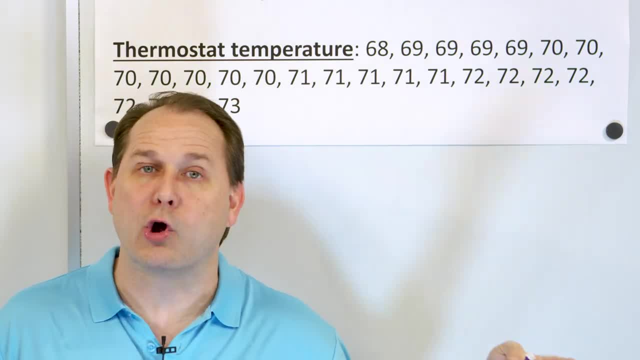 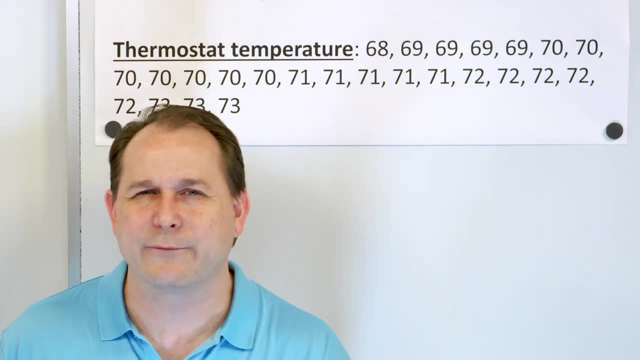 frequency that something happens. it means a higher frequency means it happens more often. So the numbers that are in here more often are going to have a higher frequency because they're more frequent. Frequent kind of means frequency, Higher frequency means higher the higher. 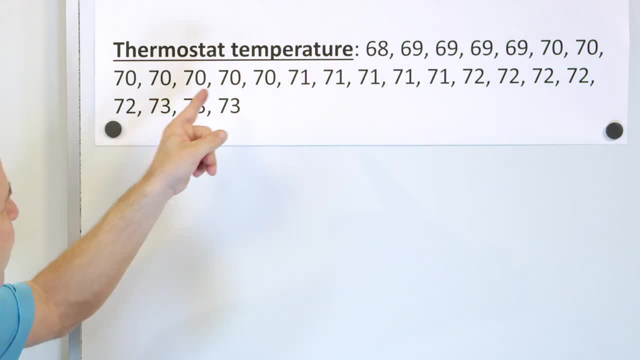 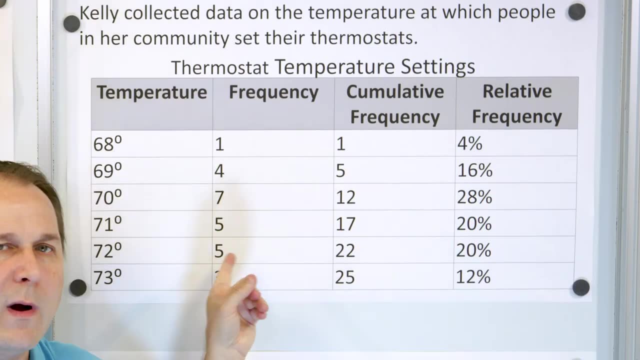 frequency that that situation is happening. Now we want to boil this down into a table. I am going to show you a peek at what we're trying to do. This is the completed frequency table. This is going to start out just by talking about this table because it's kind of overwhelming. You have a. 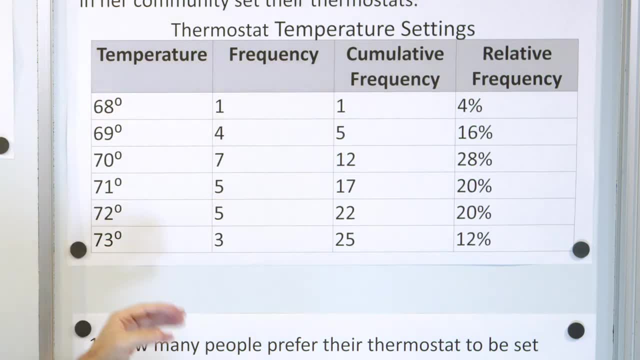 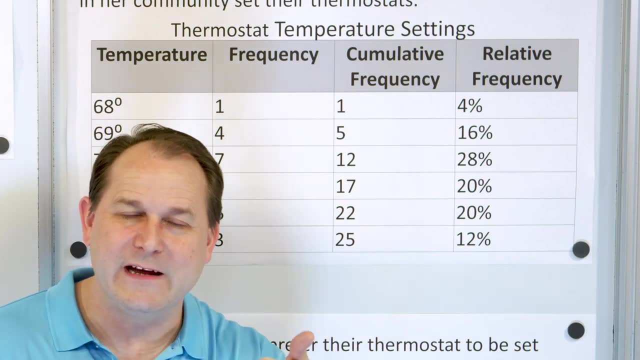 bunch of numbers over here, the temperature. We have this thing called frequency. What does that mean? Then we have something called cumulative frequency. What does that mean? And then we have something called relative frequency. So we have frequency cumulative, frequency, relative. 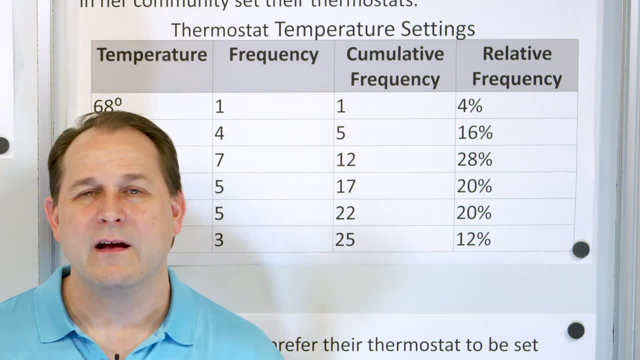 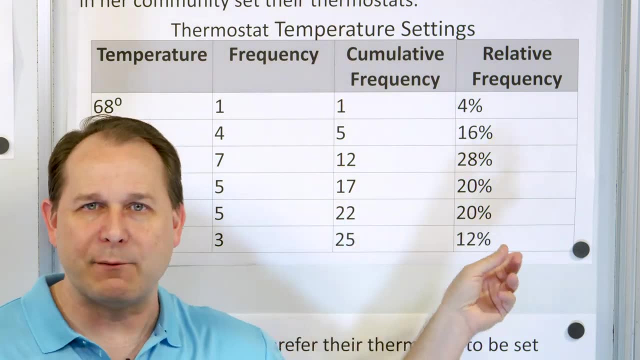 frequency, As with everything in life. once you understand the definitions, then everything's easy. So this is where we're going, Don't stress out about it. We're going to create this table right now, ourself, and then we're going to have a pretty version of it here. But our goal 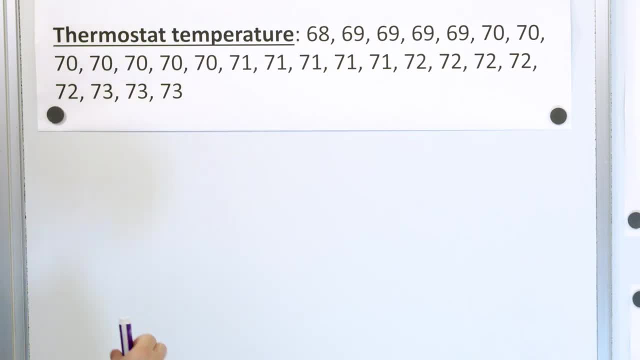 is to fill this table out. So let's go over here and let's start by talking about what this data represents. It is the temperature people want to put their thermostat at right. So what we're going to do is we're going to make a column, And the first column is going to be the temperature. 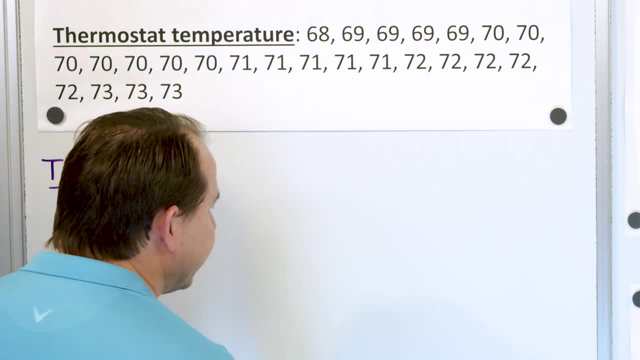 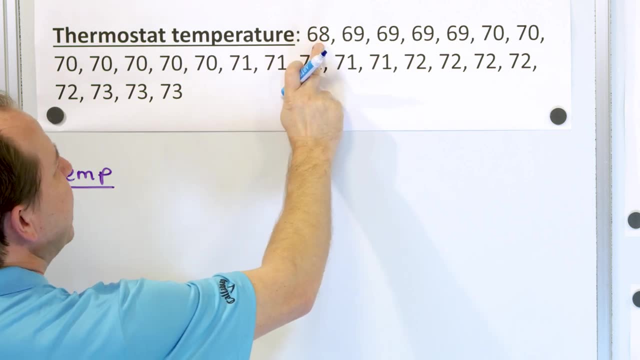 This is the temperature that people respond to us and tell them that they want to set their house at Now. we've already ordered the data from least to greatest, So you can see the temperatures from 68 all the way to 73 degrees. We don't have anybody lower than 68, and we don't have anybody. 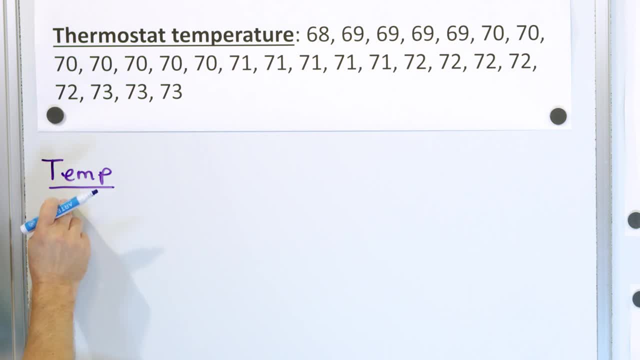 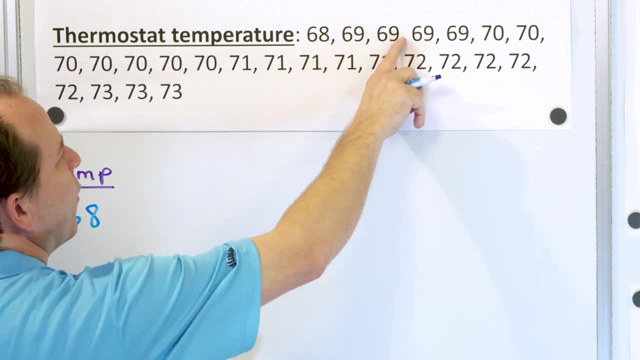 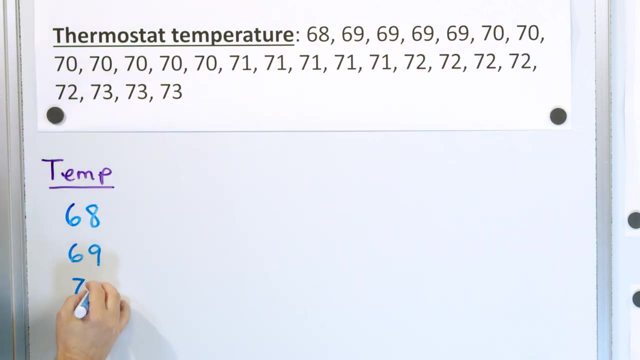 higher than 73. So all of the numbers that go in the temperature column are all of the temperatures that we got for answers. So some people wanted 68 degrees, right. Some people wanted 69 degrees, right. Some people wanted 70 degrees right here. Some people wanted 71 degrees, Some people wanted 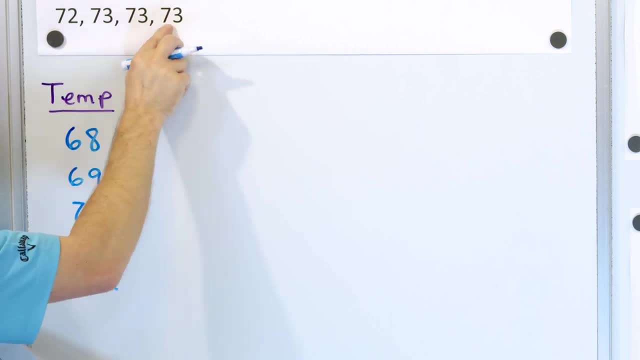 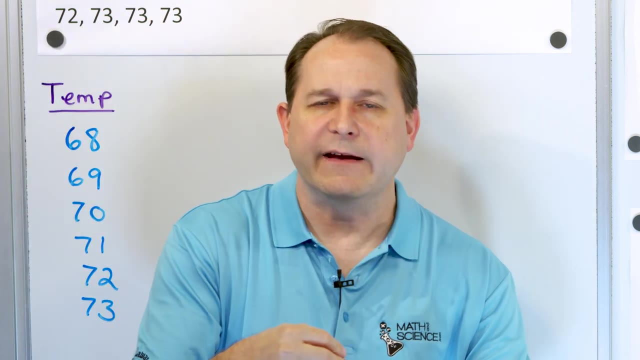 72 degrees And finally some people wanted 70 degrees, So we're going to set our house at 73 degrees. Some people wanted 73 degrees, So in the temperature column we're just listing all of the unique responses. So in this case it's all about temperature and we got numbers back. 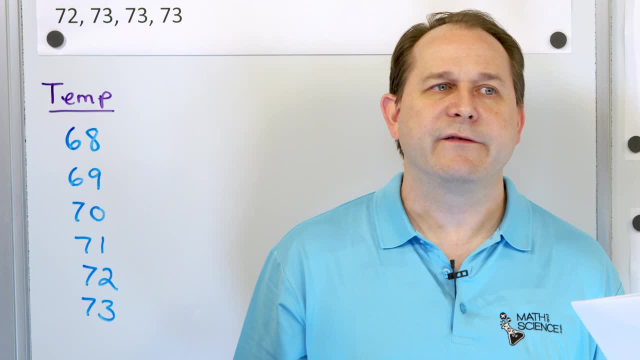 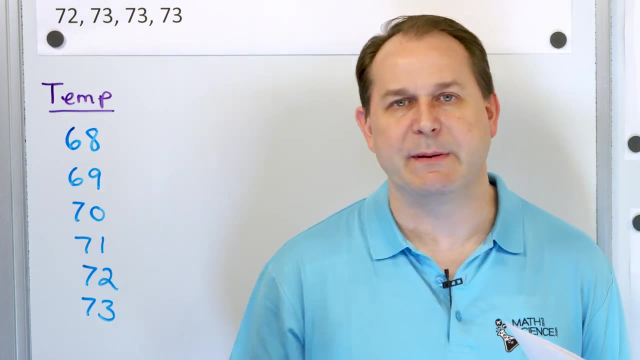 But the data could be: what's your favorite color, right? And so I ask 100 people what the favorite color is. Some people would name red, Some people would say blue, Some people would say green, Some people would say pink, Some people would say purple, Some people would say brown, Some people 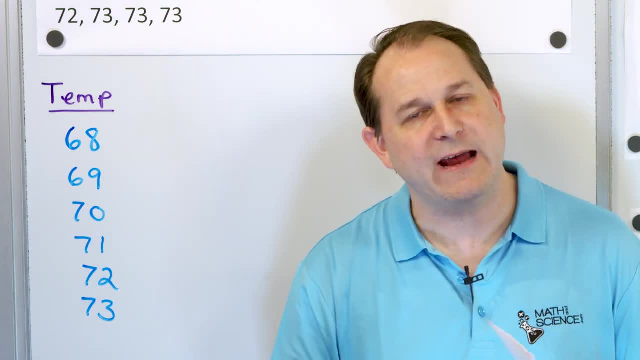 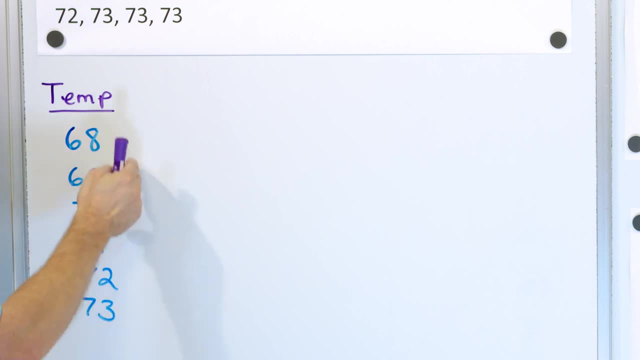 would say black, And those answers would be the ones that we would list in the table, because those are all the answers we got. Now what we have to do is we have to try to see how often people responded with these numbers. So we have. 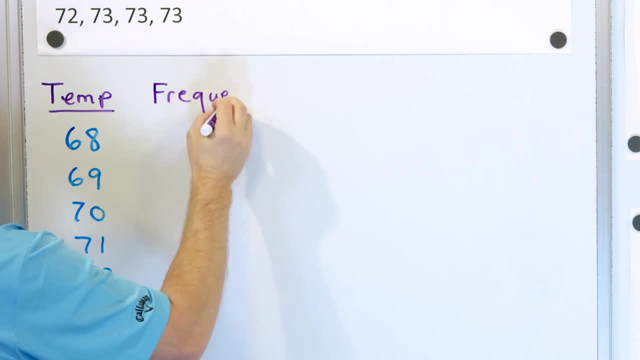 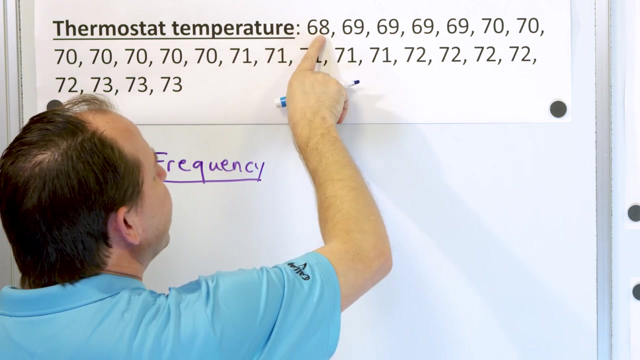 something called the frequency, right, So we have something called the frequency. Remember, the frequency is how often something is happening. So we look at the data here. in the table here, 68 degrees only occurs one time. Only one person answered that: Very low frequency. Low means it. 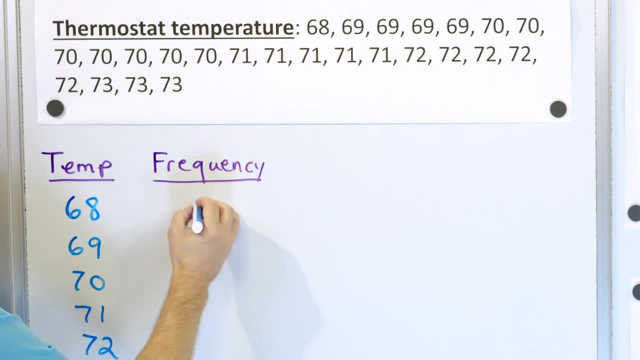 doesn't happen very often Only one person. So under the frequency column you're going to put down how many times that occurred, How many times that answer happened. And it only happened one time. Now for 69,. that happened one, two, three, four times. So we had four different houses answer 69. And then for 70,. 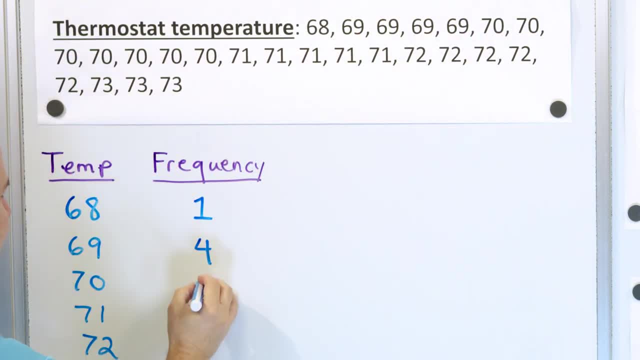 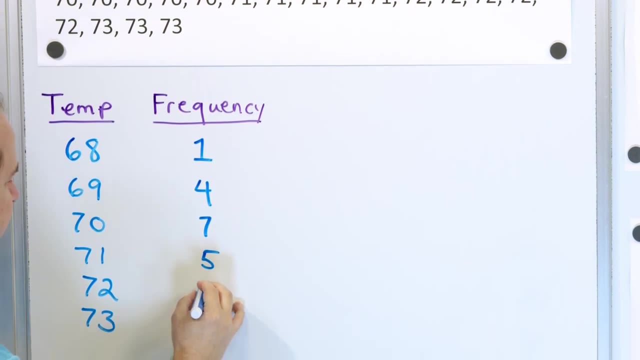 one, two, three, four, five, six. seven people answered 70. And then 71,. we had one, two, three, four, five. Five people answered 71. And then 72,. we had one, two, three, four, five answer 71.. And don't worry about this table being so pretty. 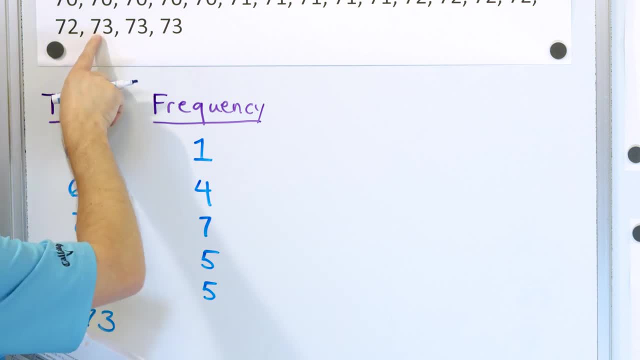 because we're going to make a pretty version in a second. And then we had 73. Only three people answered 73. So before whoops, I put the wrong number here- Not seven, it should be a three. Only three people answered 73 degrees. Now, before you do anything else, this table by itself has a 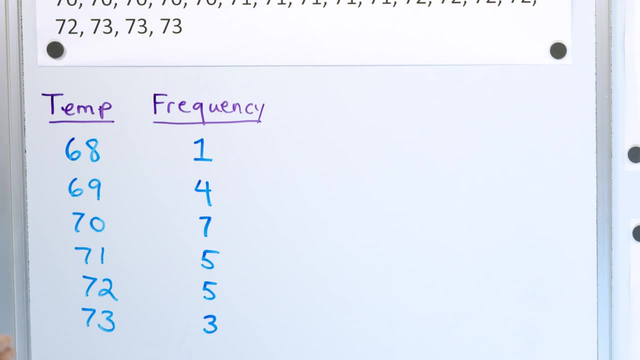 lot of value. We have one, four, seven, five, five, three, Because it's very hard to look at this data and for you to tell me, well, what's going on, What's going on, What's going on, What's. 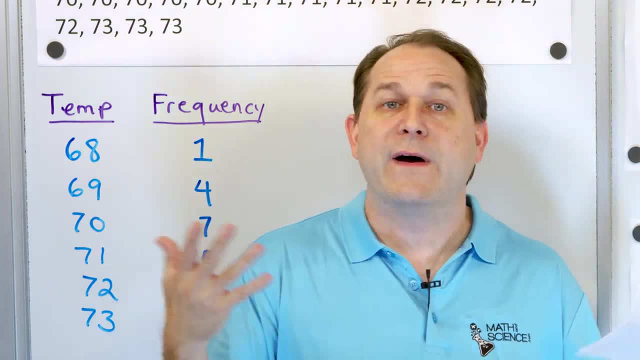 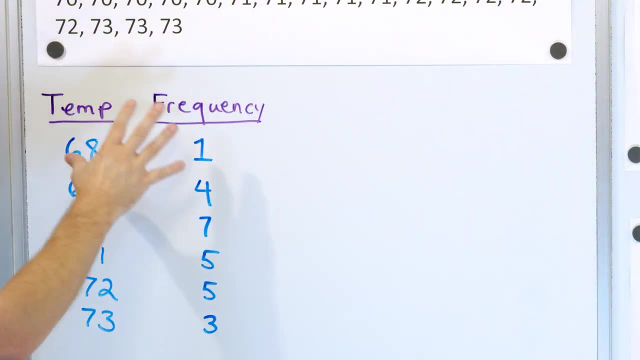 the most common temperature. I mean, you could count them, But you see what, if I gave you 500 numbers, You're not going to be able to look at all those numbers and tell what the most common one is. But if I present it in a table, all of the data is here And you can immediately see. 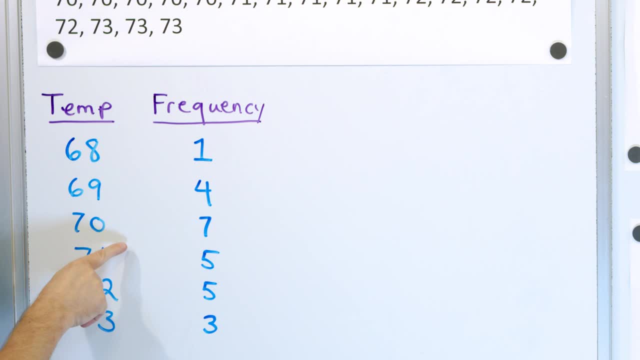 okay, the most common answer was 70 degrees. We had some people a little bit higher and some people a little bit lower, And look the farther we got away from the most common answer to 68 and to 73 degrees. then fewer people, fewer people had that setting. So that's very common. 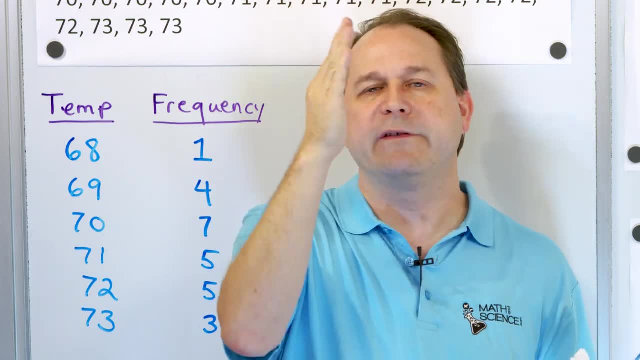 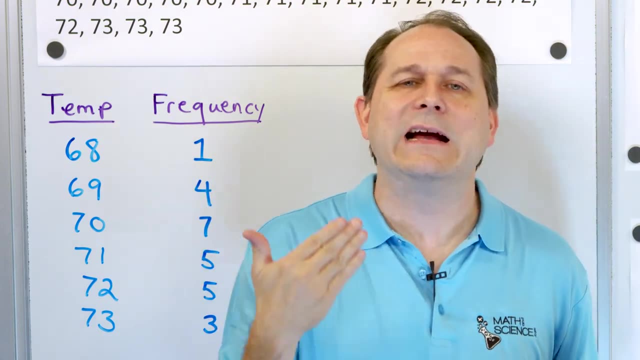 in real life. You'll have a most common answer where most of the people will answer, And then, as you go farther away from that, the frequency goes down. So remember, high frequency means high number of respondents, because it's more frequently answered, And as you go farther away, to more. 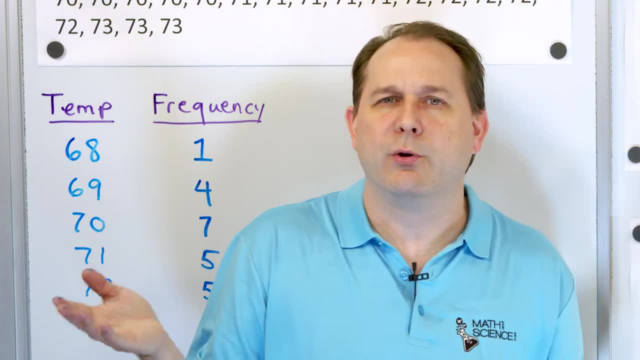 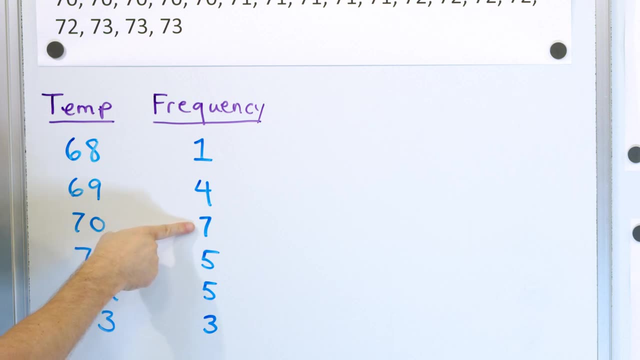 extreme cold, more extreme hot. then fewer and fewer people want to set their thermostat there. So the answer is less frequency. So we have high frequency here, a big number, and low frequency here for a small number. Now again, this table is very valuable because you can see right away. 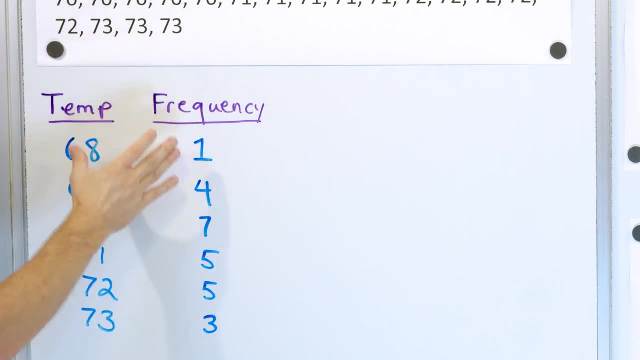 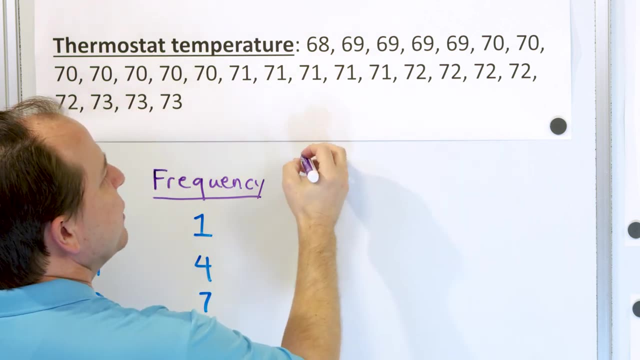 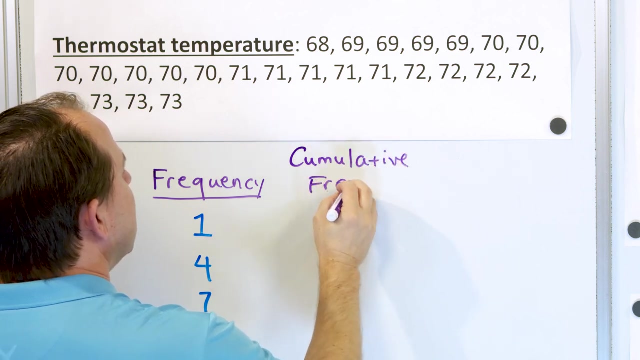 okay, this is most common. Okay, this is not so common, And it's way easier to digest this than to look at this table. All right, So the next thing we have to talk about is the cumulative frequency. Cumulative frequency, So I'm going to call it cumulative freak. 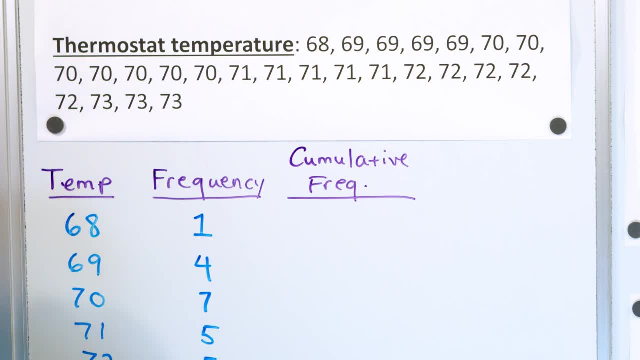 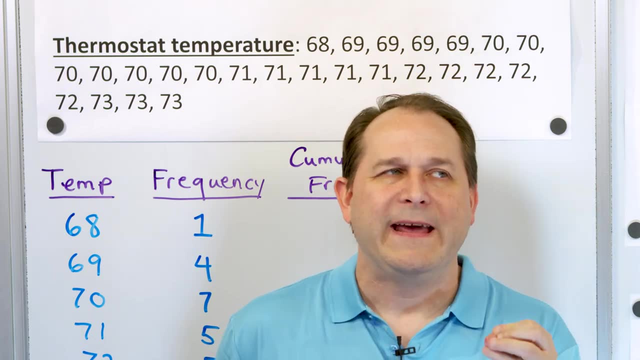 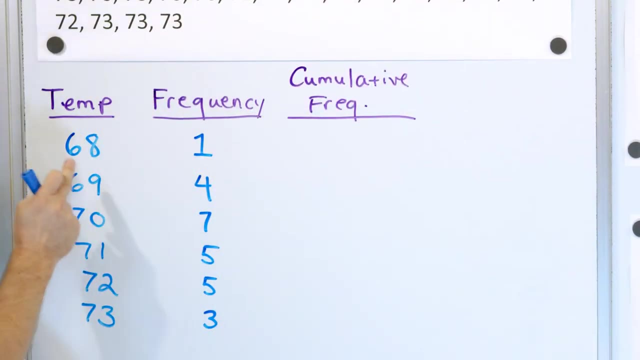 All, right Now. I'm going to tell you right now that this table, this column, it's useful, but it's not maybe The most important table in the chart. Okay, What we really want to know is how many people responded. If I ask you, because it's useful to know, we had one person answer this, four people. 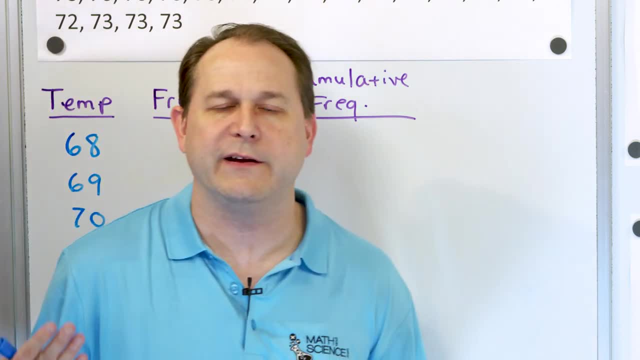 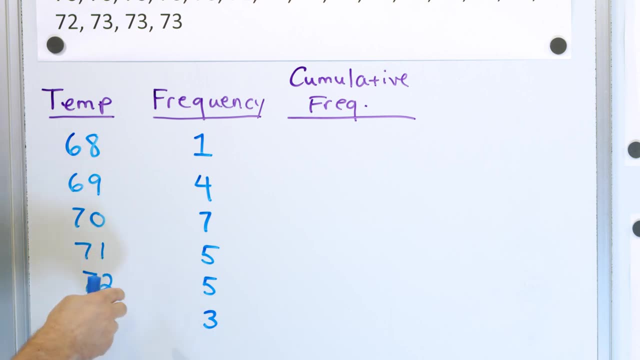 answer this. seven people answer this. It would be useful to know how many total respondents we have. So we're going to add them all together And we can add them all together And we can see in this case that we're going to get 25, because this is 10, right, And then this is 10 more. 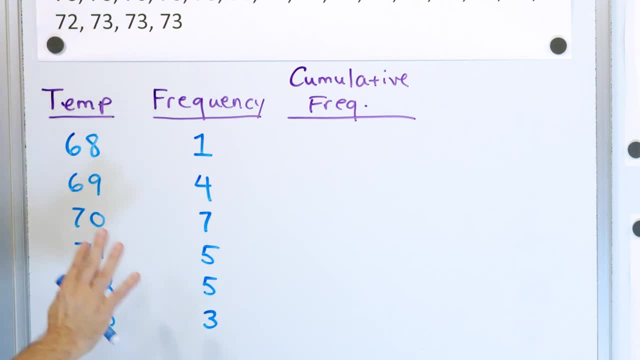 that's 20.. And then that would be 25.. So there's 25 respondents all together, But the cumulative frequency just makes it a line entry where we start adding up all of the people that answered, And that's why it's called cumulative Cumulative. 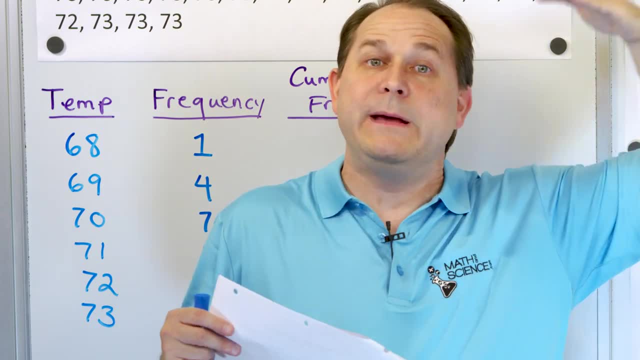 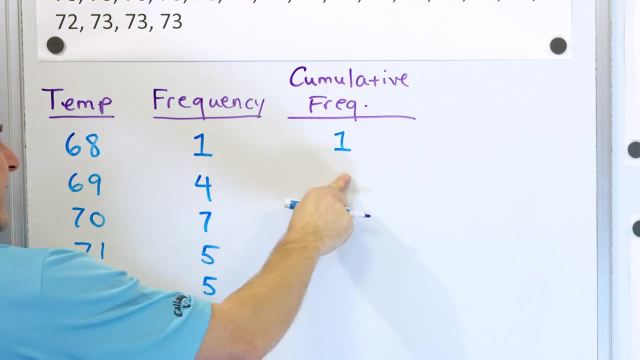 means you add as you go. So in that line of the table how many people have answered up above. So the cumulative frequency for the first line is just one person, because there's only one person here. But in this line what you answer is you say how many people answered before you. 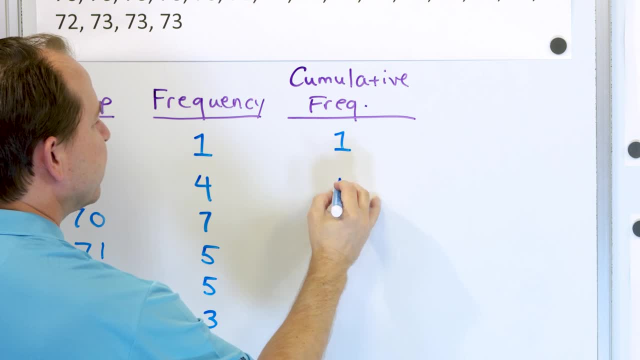 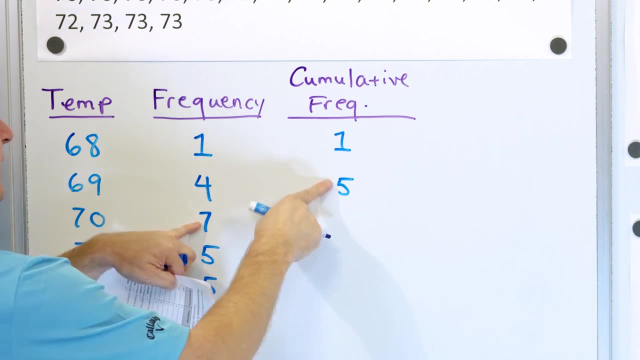 plus how many new people answered, for a total of five. So the cumulative frequency right here is 22.. And then for this line you say: well, seven more people answered and five. you add these two together. This is how many answered before. Seven more is going to give you an answer of 12.. So 12. 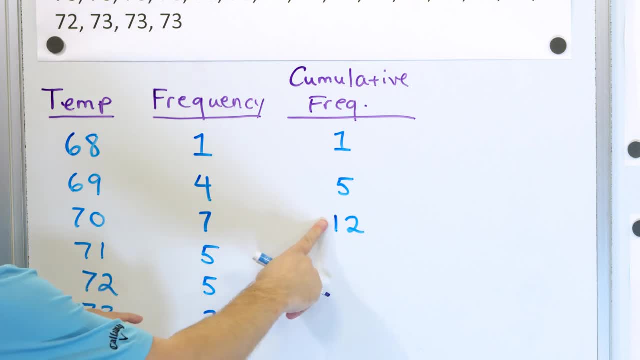 goes right here in this column, And then for this line you say how many people answered before plus how many new answers. 12 plus five is 17.. So 17 goes here, And then for this one we just add these: How many people answered before and how many people are answering at this. 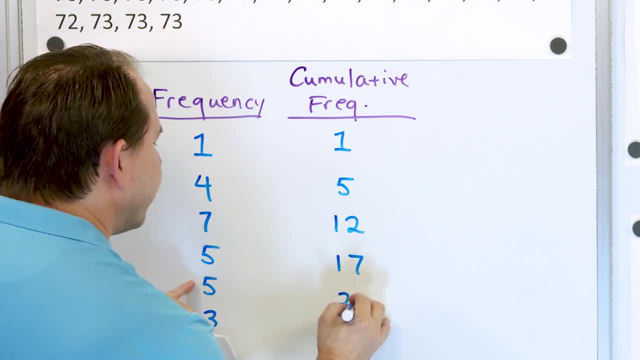 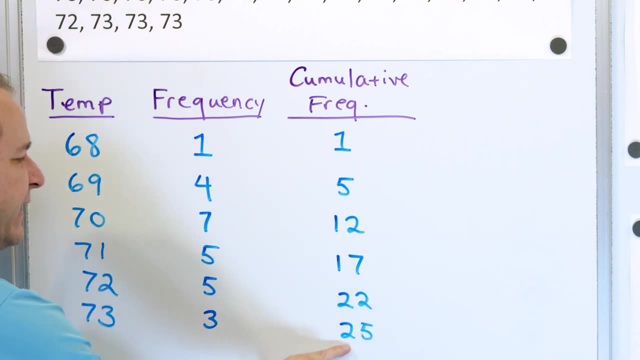 number 17 plus five is 22.. And then finally, 22 plus three is 22.. So that's how many people answered before 25.. Notice that basically, the very last entry in the table is telling you how many data points you have, how many people you have. Now. this is the most important. number 25 is the most. 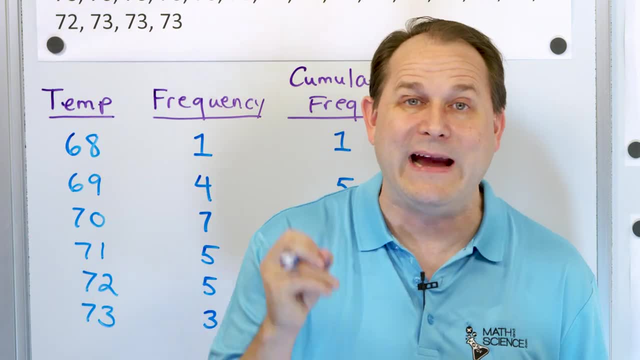 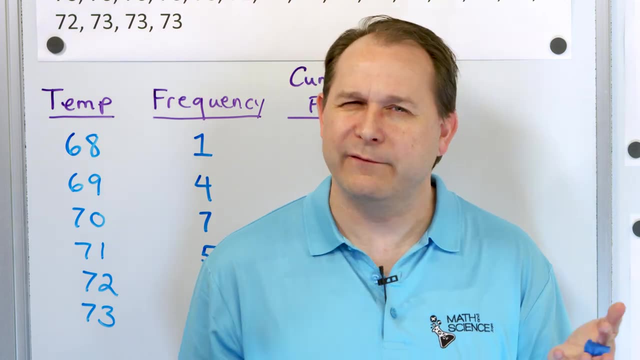 important number because it is telling you how many people answered your survey. That's important because you need to know: did a thousand people answer or did two people answer? I mean it's really important, right? So you need to know how many people answered. We just put a line item in. 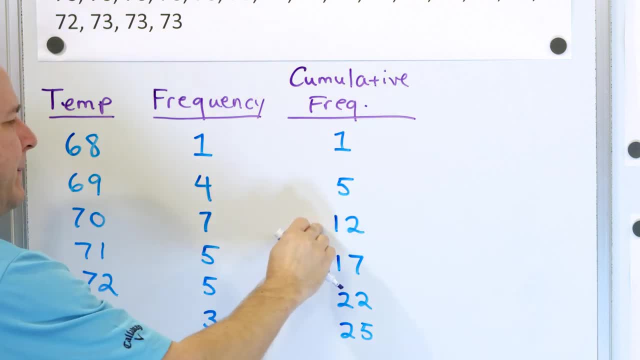 the table. So we say at each little row it tells you how many people answered above this, including this. So it's like seven plus the five that answered before Here is five plus the 12 that answered before Here's the five plus the 17 that answered before Here is the three. 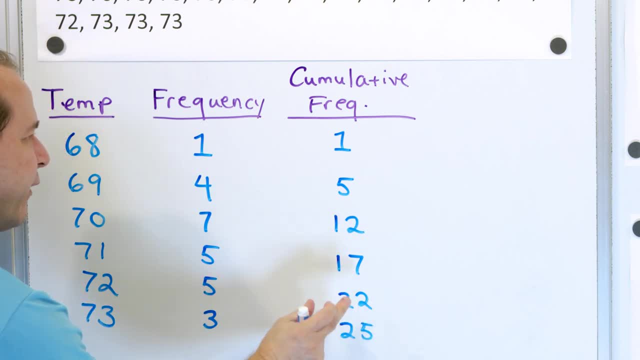 plus the 22 answered before. So the very last entry is always going to be the cumulative, which is the total number of people who answered. So frequency means how many people answered a certain thermostat setting, And cumulative is just adding them all up down in the table. 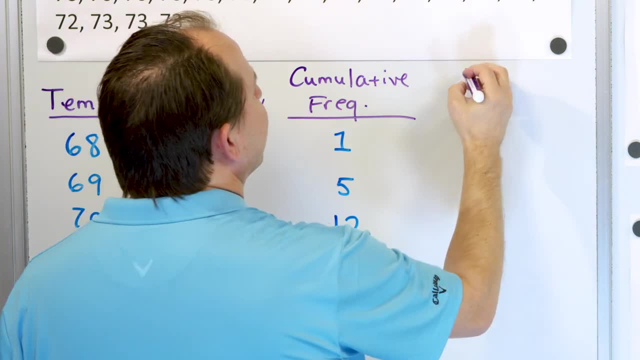 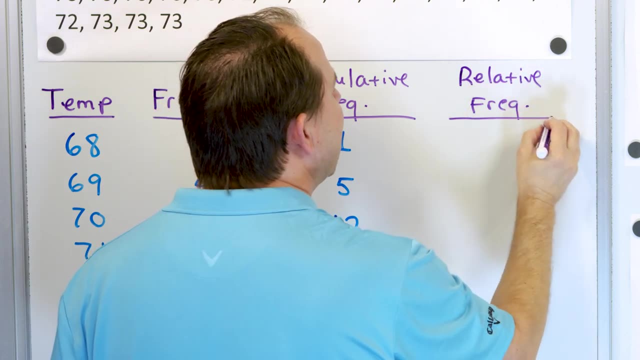 All right. Now the last thing we need to do is talk about something called a relative frequency, And this one's actually probably, in my opinion, the most important entry in the table, So it would be nice. I mean, this is useful. Okay, You can look. 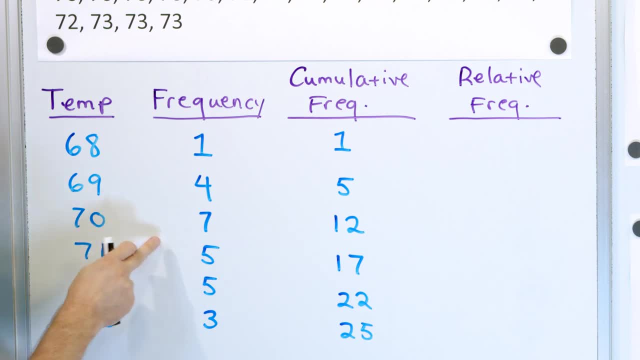 at the frequency You can say: oh, most people chose 70.. Oh, there's some people that chose 71.. A very few people chose 68.. Okay, That's useful, But wouldn't it be more useful to express it as: 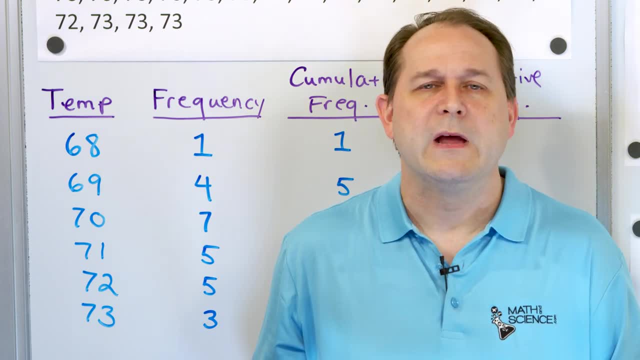 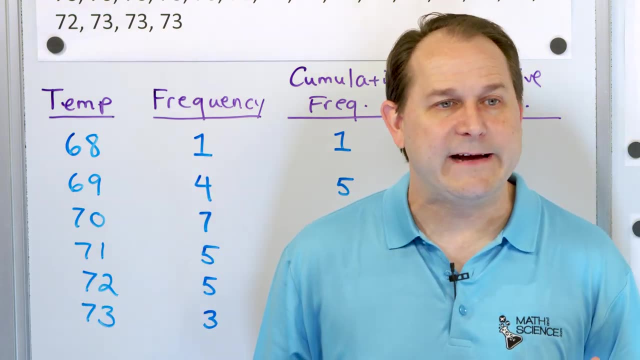 a percentage. A percentage is really, really useful. What if I told you that you took all the data in the neighborhood of all the temperatures everybody wanted to set And then I said: 30% chose, 70 degrees, 60% chose, or whatever? 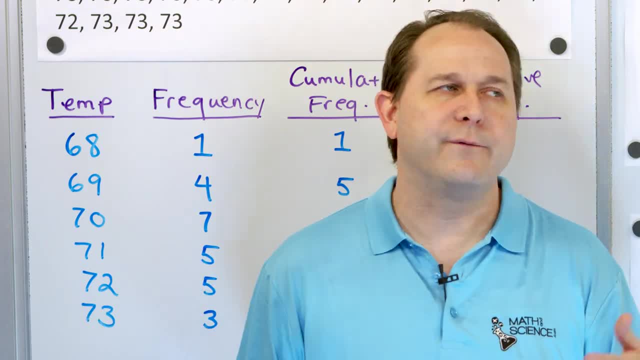 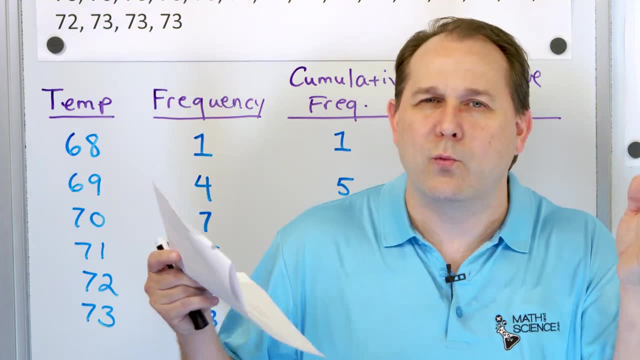 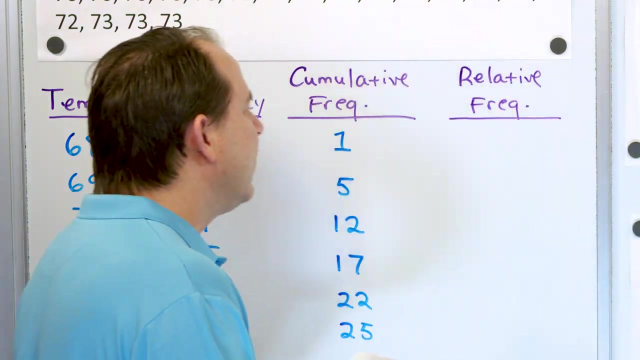 60% chose you know 72 degrees and 40% chose a different temperature. Then you would know right away, because you know 60% of the people, that's a majority. You would know right away, without having to dig through the data, what most of the people actually indicated here. So what we want, 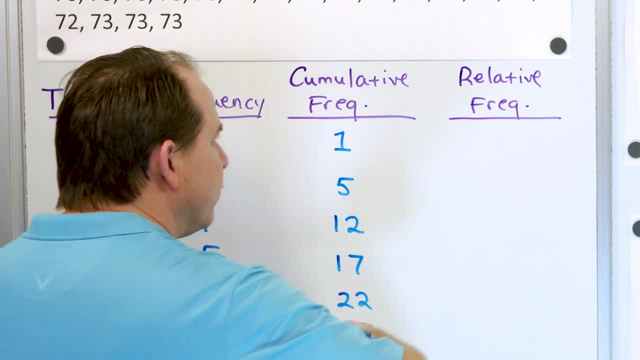 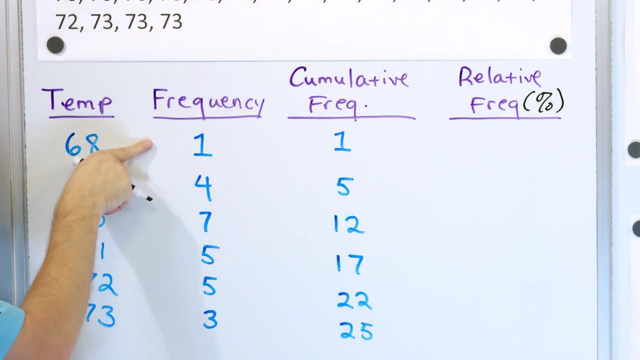 to somehow put in this column is a percentage, So it's a relative frequency, but I'm going to put a parentheses here. This is a percentage. We basically want to know: what is the percentage of this answer compared to the whole thing? That's really what we want. 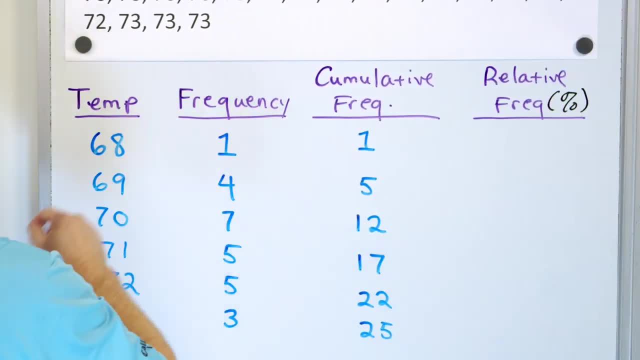 to know. So I'm going to back this table over here and we're going to calculate this here. So for this first line, only one person said that. they answered that they want 68 degrees, But there's 25 respondents, Remember 25 respondents total. So 1 out of 25, that's the percentage of people that answered this entry. 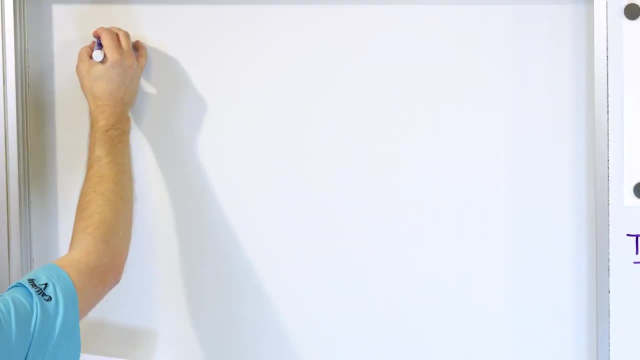 68 degrees of 25.. So if you go over here and you say 1 out of 25, that is 1 divided by 25, right, And 1 divided by 25 actually works out to be 0.04.. Just divide it long division or run it through a. 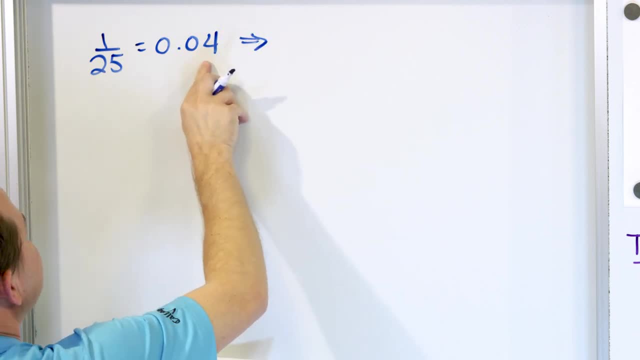 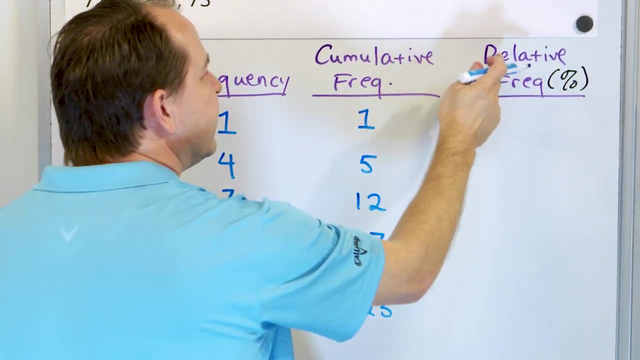 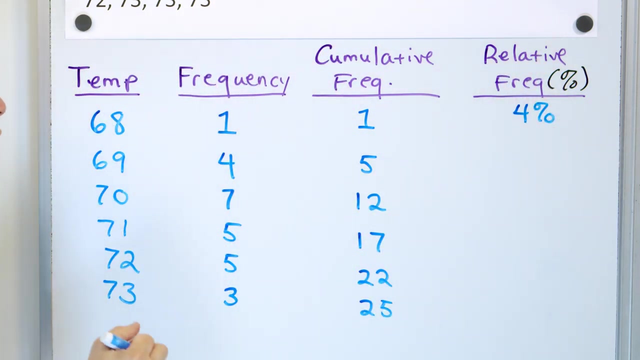 calculator And if you put that as a percentage, you multiply by 100, move the decimal, that is 4%, 4%. And so what that does is you come over here and say the relative frequency as a percentage is 4% And without filling out the rest of the table, you know immediately that 4% of the people 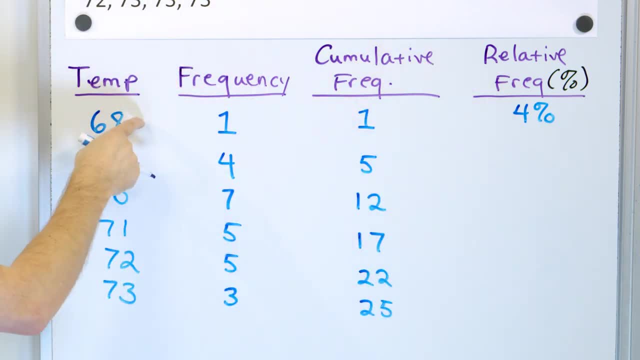 that answered this survey in your neighborhood actually wanted this temperature, And we expect the numbers to go up from here because we had more respondents here, So let's take a look at this one. There were four people that wanted 69 degrees out of 25, 4 out of 25.. So we can go here. 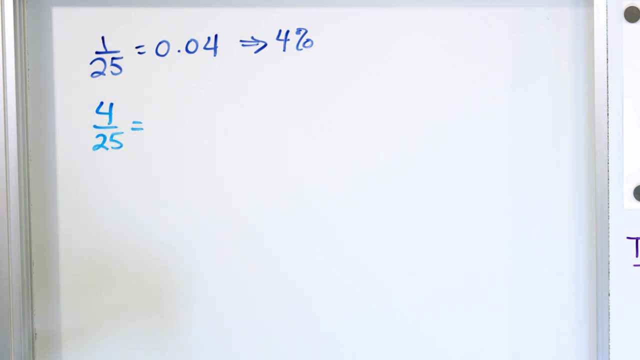 and say what is 4 divided by 25, or 4 out of 25? And 4 out of 25 is 0.16.. And if you convert to a percent, move the decimal two spots, 16%. And so we come over here and we say 16%, All right. 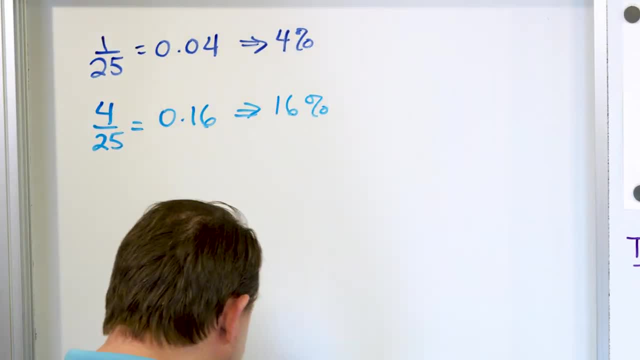 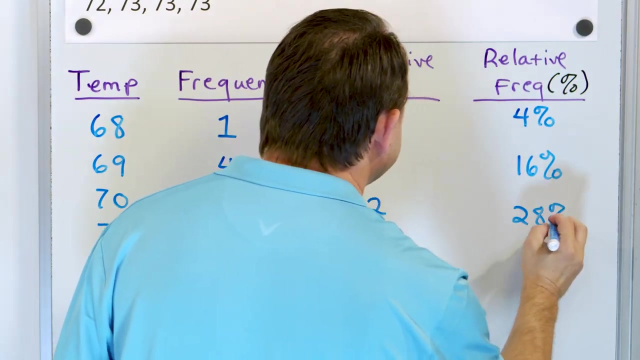 How many people answered: 70 degrees. Seven people, 7 out of 25.. So you say 7 out of 25, 7 divided by 25 is 0.28. And as a percent move the decimal you get 28%, 28%. So 28%. Here we had five people. 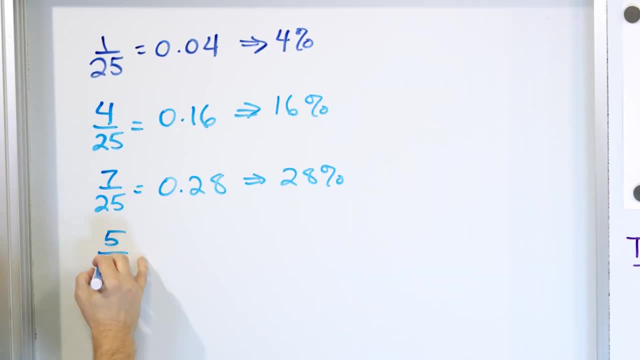 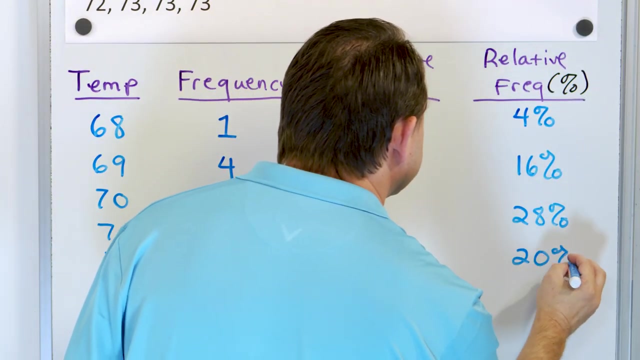 answer: out of a total of 25.. So 5 out of 25. That's going to be 0.2. when you do that division And when you multiply by 100, decimal moves two positions to 20%. So what do we put here? 20%, And then this is the same number. 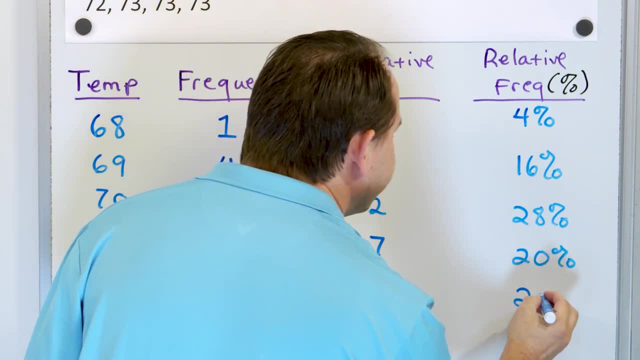 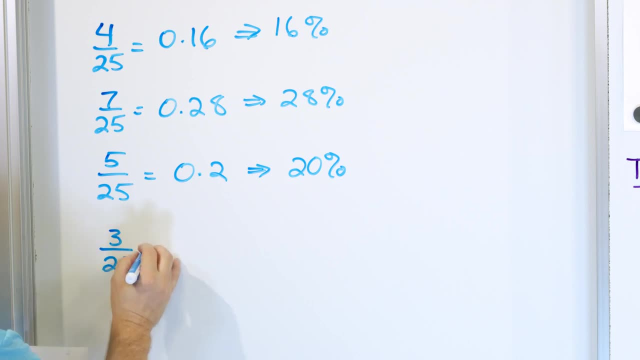 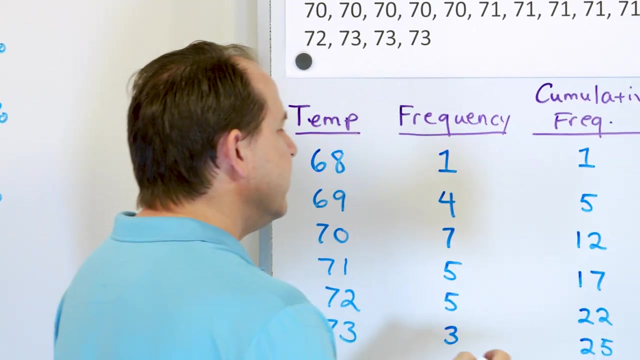 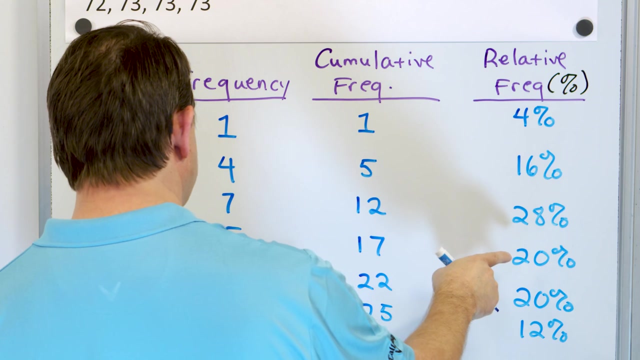 of people answered as this. So this is 5 out of 25 also, So it's also 20%. And then, finally, we had three respondents here And 3 out of 25 works out to be 0.12.. Which is 12%. Just move the decimal two spots So you get 12%. So we have 4%, 16,, 28,, 20,, 20, and 12.. 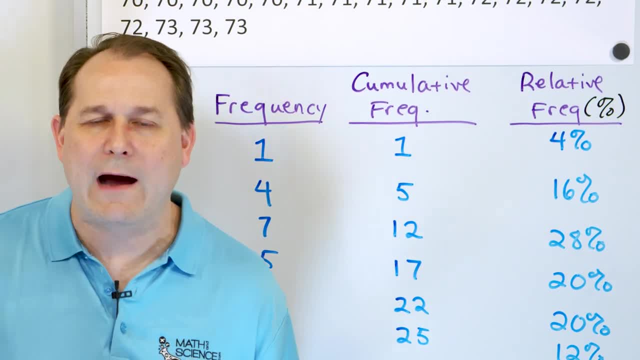 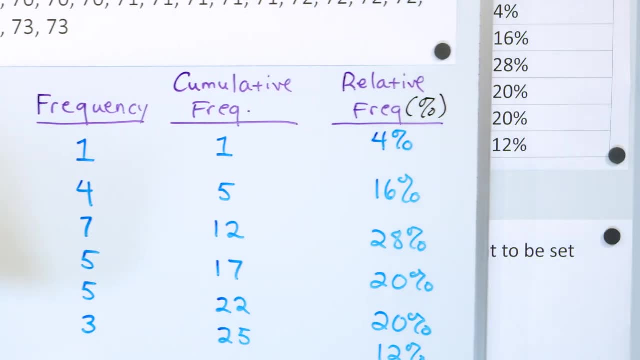 Now this is our table. Now that we've built it ourself and you know how it's constructed, let's go look at the pretty version of it, which looks a little overwhelming until you see how it's done. So these numbers, unless I made a mistake, are exactly the same as these. I'm just 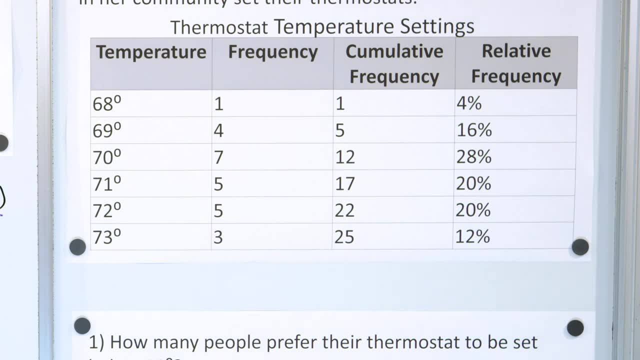 going to take a look real quick: 4,, 4,, 5,, 16,, 7,, 12,, 28,, 5,, 17,, 20,, 5,, 22,, 20,, 3,, 25,, 12,, and then 68,, 69,, 70,, 71,, 72,, 73. Here. 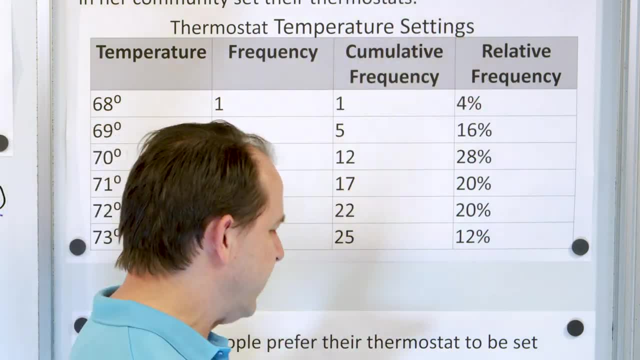 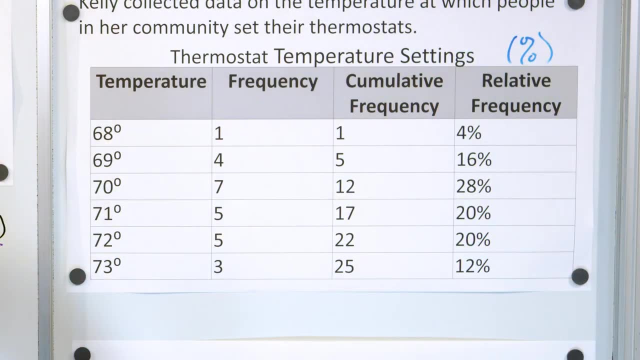 it is Temperature frequency, cumulative frequency, relative frequency, And I'm going to remind you that this relative frequency is a percentage which you can see because of all the percent symbols there. I want you to notice that this is basically telling you that the reason 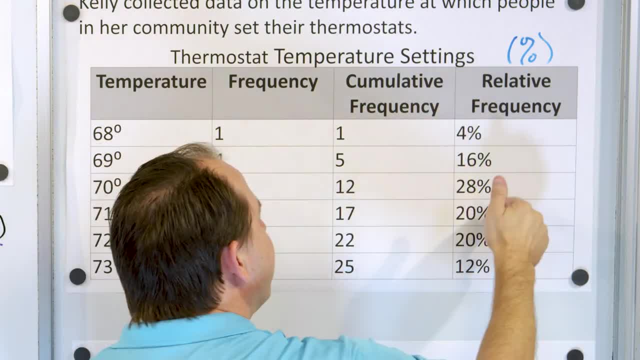 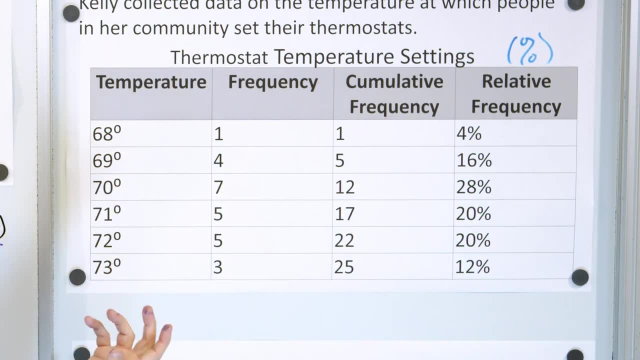 it's called relative is because it's telling you, compared to the whole, how popular was the answer. How many respondents did we get? We had 28% of the people choose 70 degrees, which is the majority answer, So it is the highest percentage. We had two separate entries for 20%, each 20%. 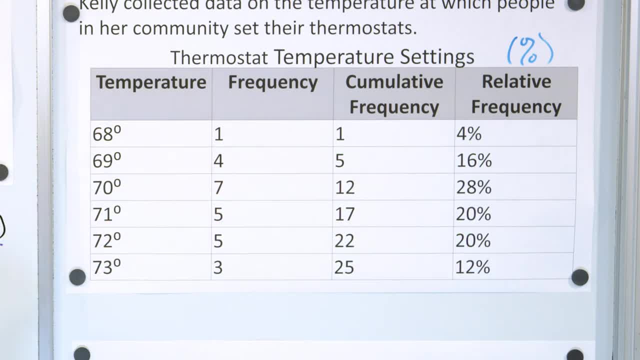 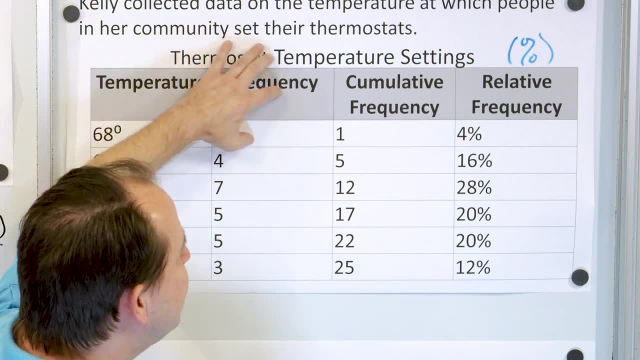 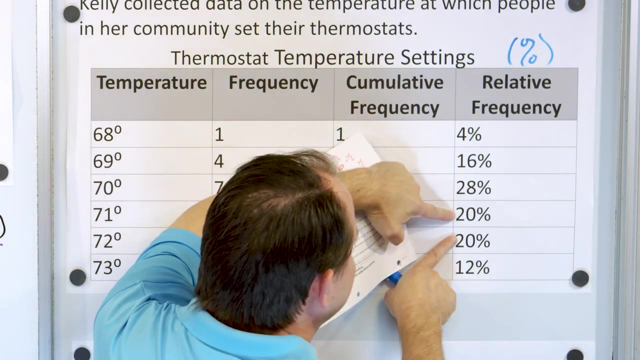 answered 71 degrees. 20% answered 72 degrees, A smaller amount answered 73, and the least amount, 4%, answered there. Now, what do you think is going to happen if you add up all of those relative percentages? They should add up to 100, right? So if you do that, 20 plus 20, that's 40. 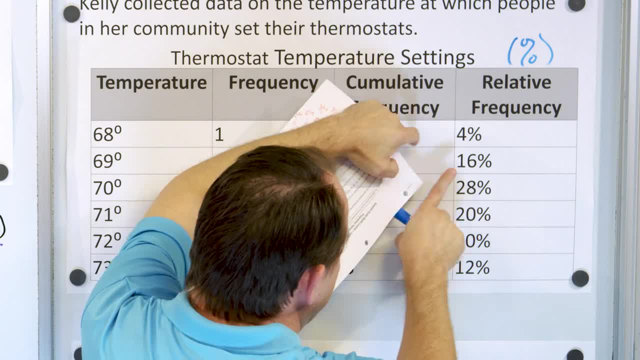 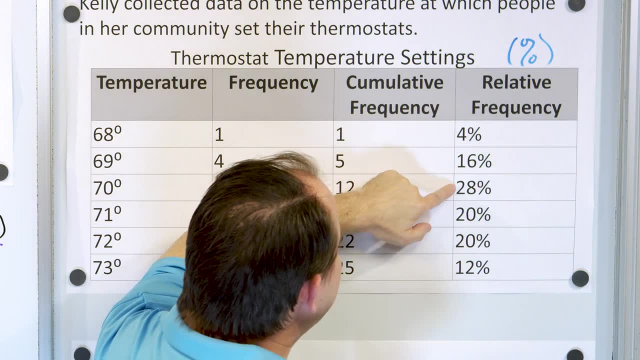 And then 16 plus 4, that's another 20.. So here you have 40,, and then you have 60 here, And then you have so 70,, 88,. you have 88 there, and then 90, and then 100.. One more time, that's 40. And 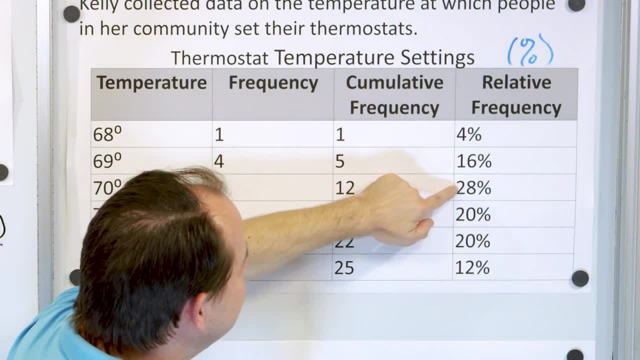 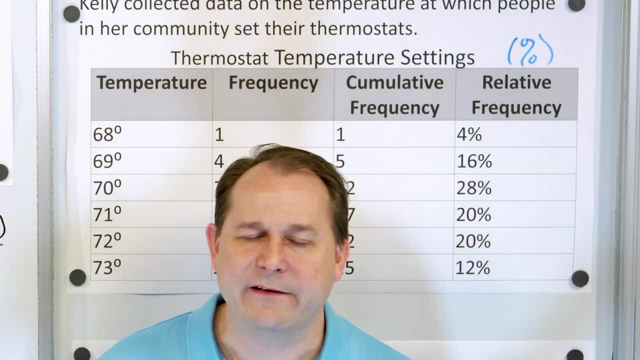 then this would be 50,, 60,, 70,, 88,, that's 88. And then 88 plus this is 90, and then 100.. So the percentages add up to 100, which they should, because after everybody answers the total. 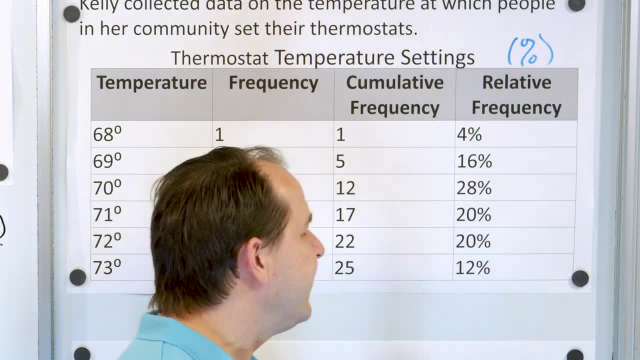 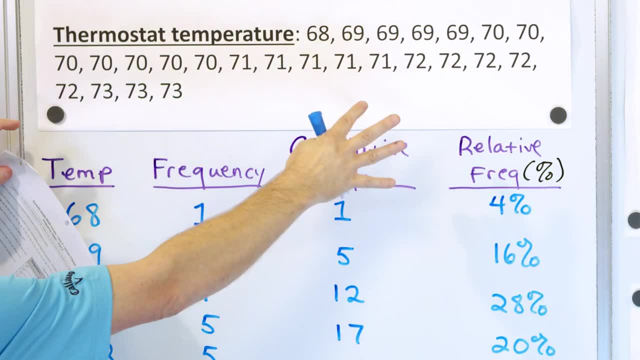 percentage of everything that we collected should add up to 100. So if you do that, then you have to add up to 100%. So this is a frequency table. It tells you at a glance, in a much more digestible way, how to interpret the data, Instead of looking at this and you don't know anything. 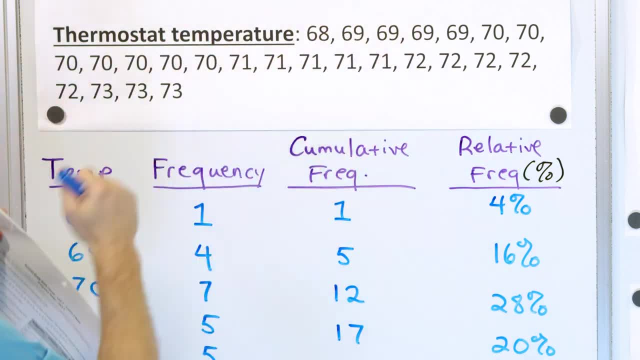 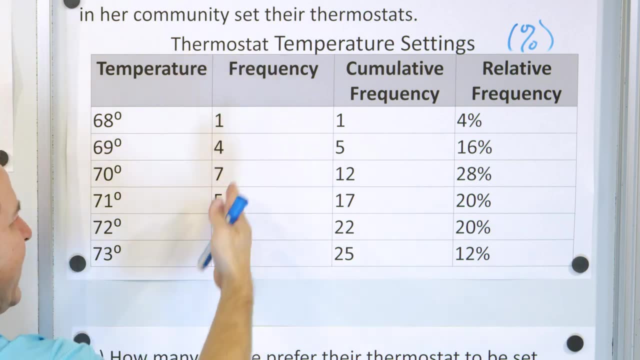 about it. you're trying to figure out what was more common, who answered what. It's basically impossible. You can look at this and say, okay, well, the people that answered 69 degrees- 16% of them answered that, And here was the number of people that answered. It's just a way easier way. 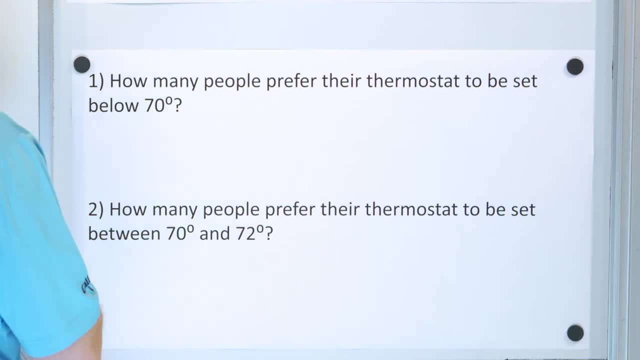 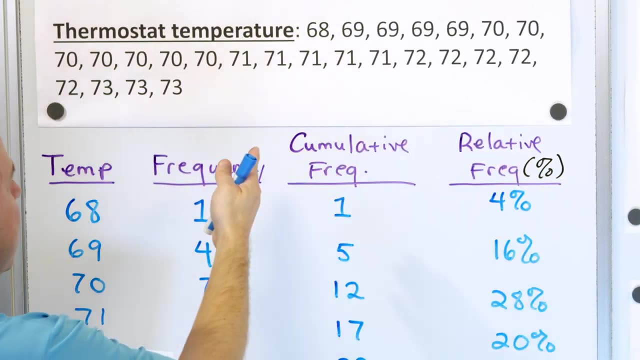 to do it. So let's take a look at problem number one. How many people prefer their thermosets to 70, below 70?? If you look at the raw data, you'd have to go over here and you'd have to say below: 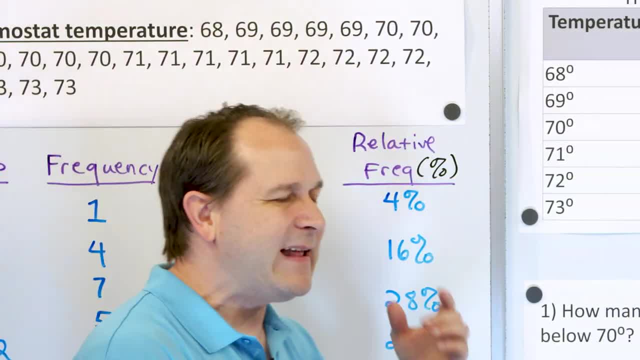 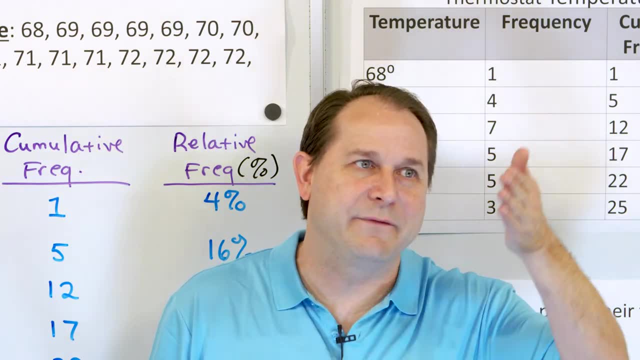 70 is everybody here and you'd have to count them. And that's kind of easy to do in this problem because there's only 25 answers. But what if I gave you 5,000 answers? Then you'd have to count them in the raw data. You can't do, you're not going to do that. A frequency table. 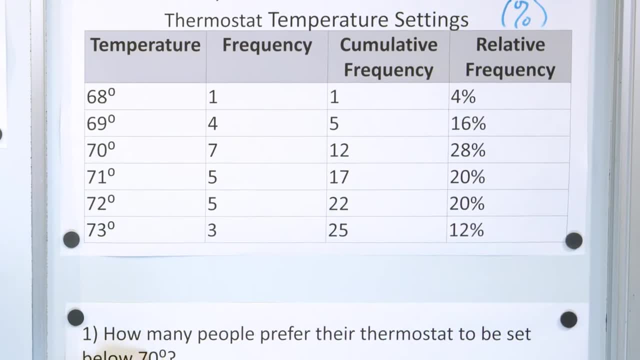 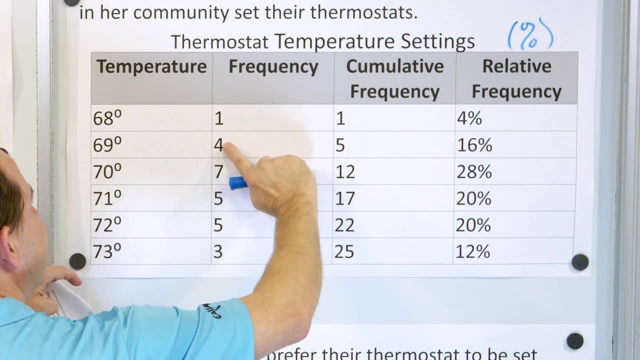 is better. How many people prefer their thermostat set below 70?? That doesn't mean 70. That means below 70, everything below. Then you just say: four people wanted it at 60% And then you'd have to count them at 69,, one at 68. You add them together, The answer is five. How many people below 70?? 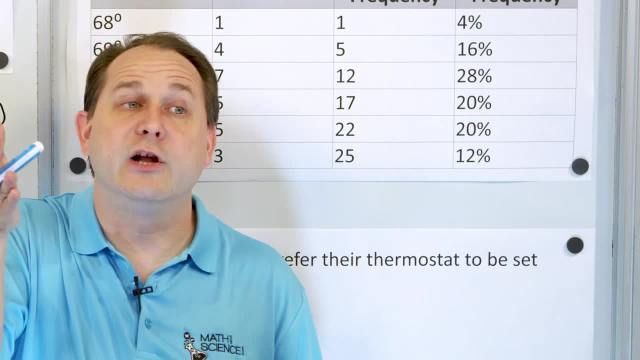 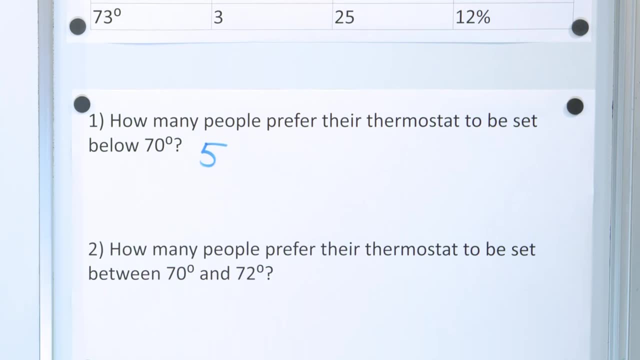 Five. Now, when you say below 70,, it does not mean 70. It means lower than 70. So we do not look at the 70 row, We look everything below that. Problem number two: how many people prefer their thermostat? 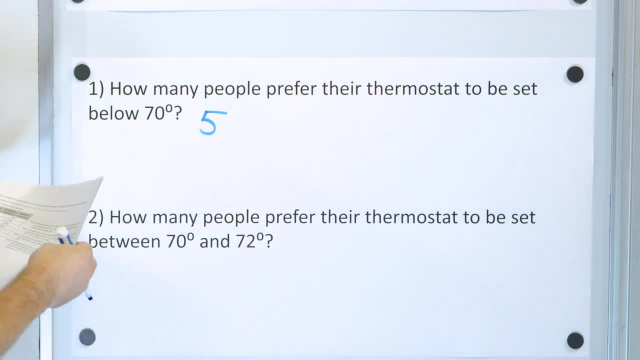 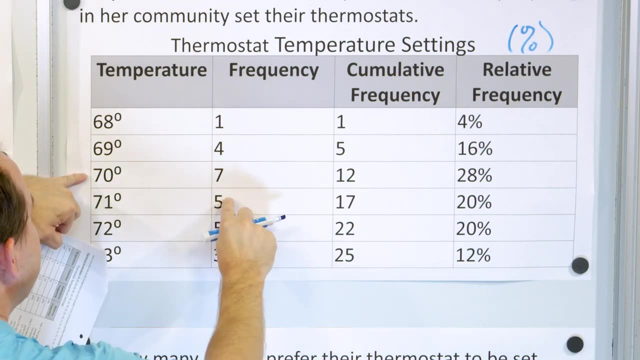 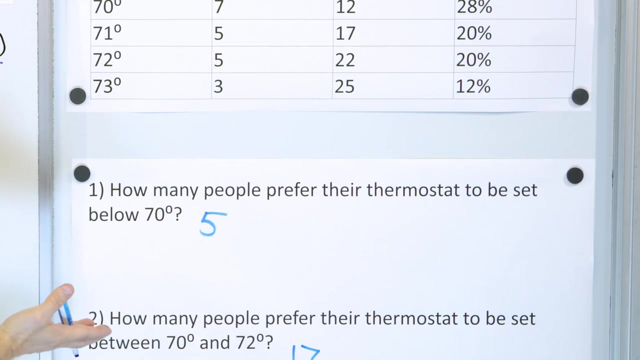 to be set between 70 and 72? Between 70 and 72. So between 70 is right here, 72 is right here. How many prefer You? just add these numbers together. This is 10.. More is 17.. So answer: 17 people prefer between 70 and 72 degrees. If you had to do this with 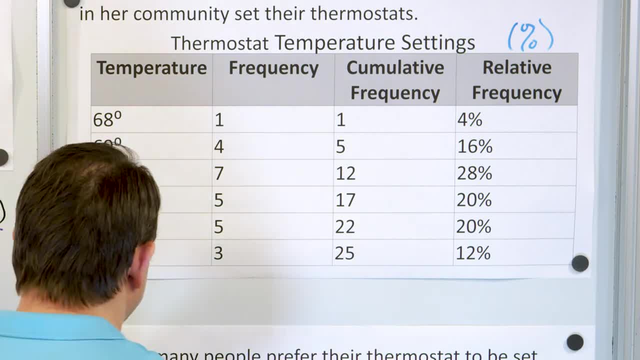 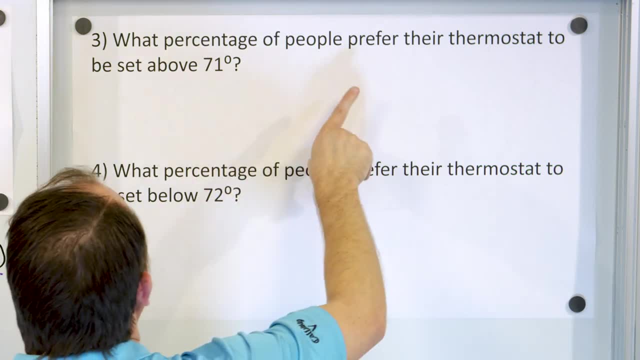 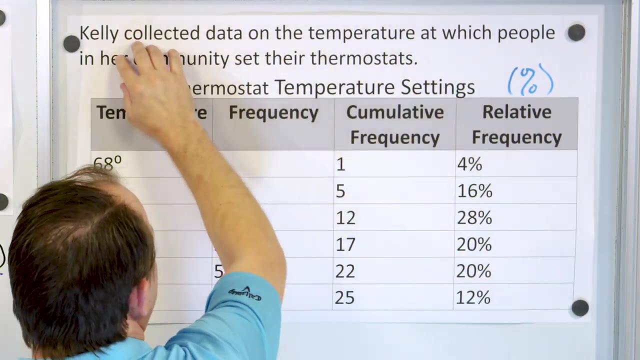 raw data you'd have to count them, But here in the table it's just much, much easier to get the information. Problem number three: what percentage of people prefer their thermostat to be set above 71? Above 71. That doesn't mean 71 degrees, That means anything higher than 71 degrees, And you 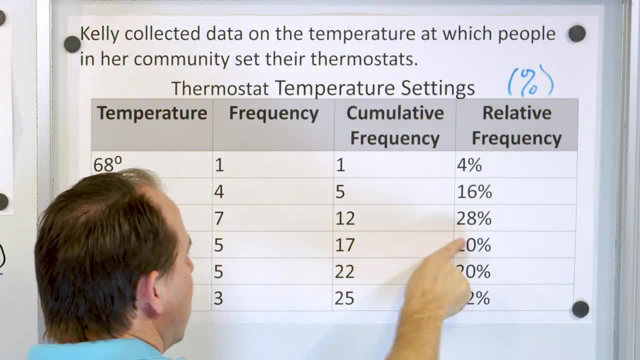 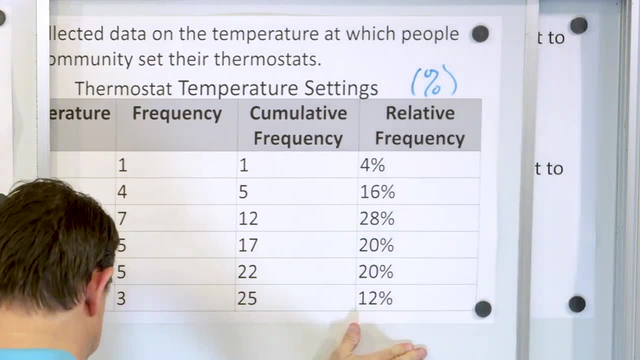 want the percentage higher than 71 degrees. Here is 71. We don't want that. We want everything above that. So we add these numbers up: 20 plus 12 more 32.. 32%. So what percentage wanted above? 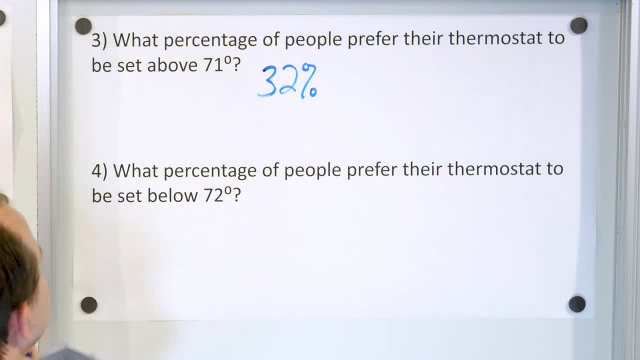 this guy: 32% prefer to be above 71 degrees. What percentage of people prefer their thermostat to be set below 72?? Not at 72,, but below 72. Here is 72. You do not want this line. You want everything. 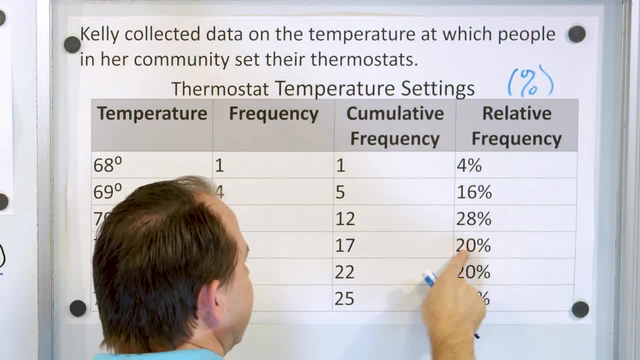 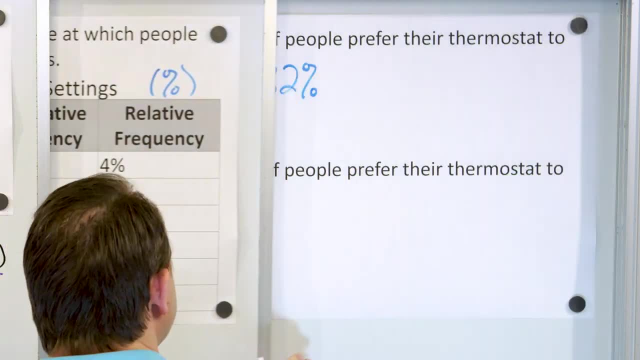 below that. We want to add up these percentages. You have 20,, 30,, 40,, 8. That's 48. And then these are 20. So 58,, 68%. So you add these guys up, you get 68%, All right, So. 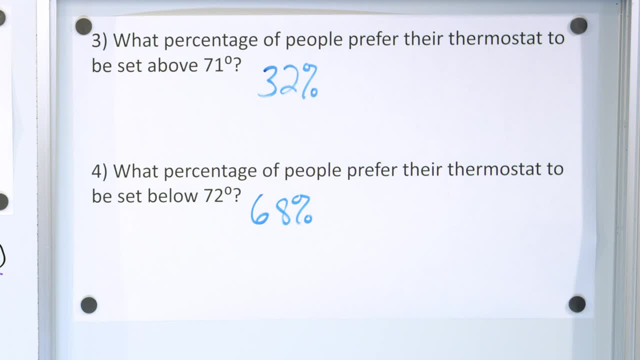 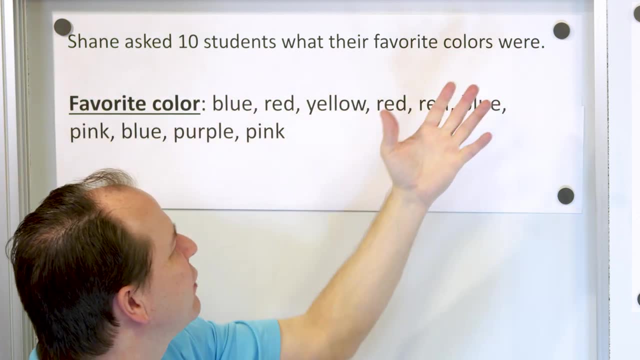 that is the first problem. We're going to take this down. We have one more and then we're going to wrap up this lesson. All right, Here is problem number two. It says Shane asked 10 students what their favorite colors were. So you have 10 answers: 1,, 2,, 3,, 4,, 5,, 6,, 7,, 8,, 9,, 10 answers And of. 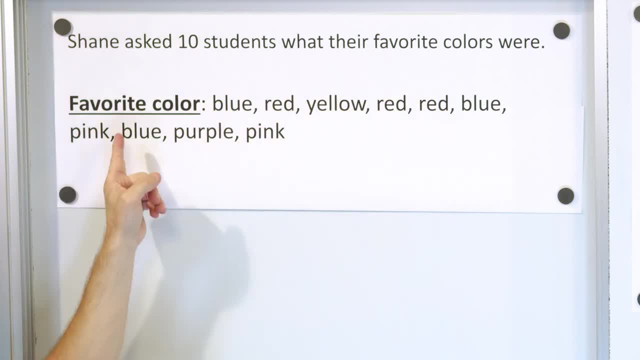 course, we have a lot of different colors that we have here. We have blue, red, yellow, red, red, blue pink, blue, purple, pink, So we have lots of different answers here. Now, if I asked you what? 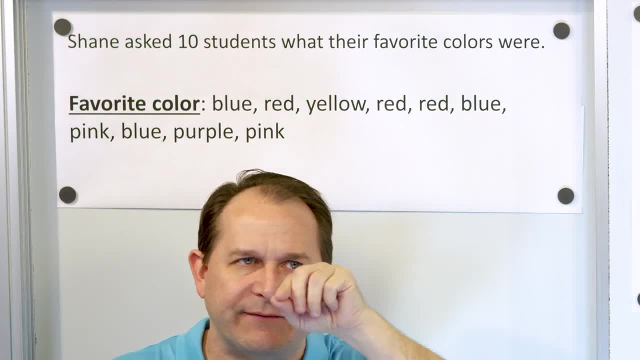 percentage of people like red. just by looking at the data you could calculate it, but you'd have to count everything. It's just hard, especially if the data is a large set of data, to look at the data and understand what it means. What is the most common color? What is the least common color? 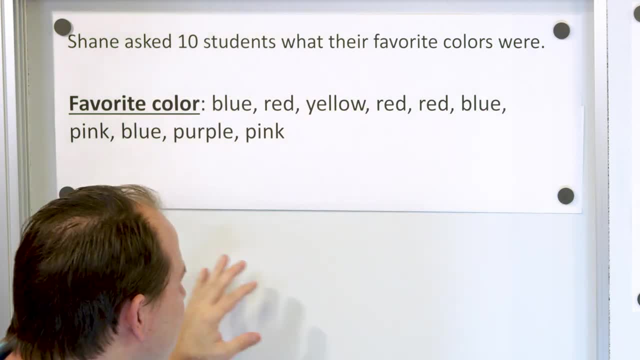 Yes, you can get it from looking at it, but it's difficult. So let's make a frequency table Now. we could draw it and calculate it like we did, But I think, now that you know, we're going to be able to. 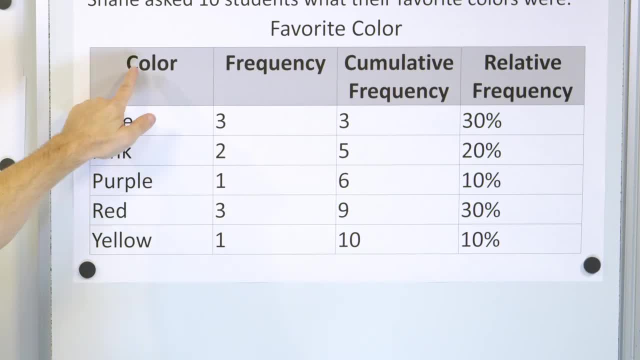 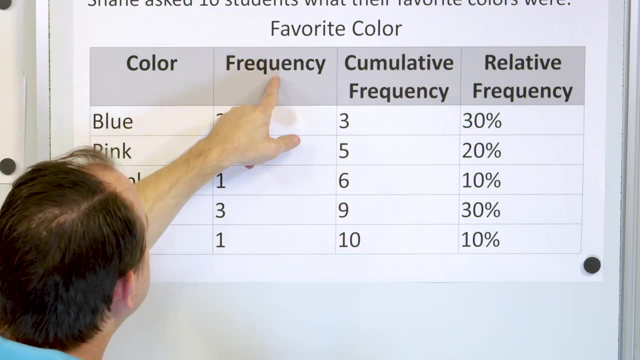 know how it's laid out. we can go straight to the finished product. We have the color, This is mean the answers that we got. We have blue answers, pink answers, purple, red, yellow answers. Now we have to create the frequency here. How many people answered blue? Well, we have 1,, 2, 3 people. 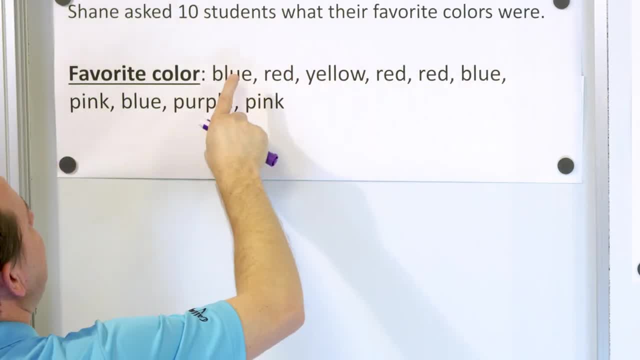 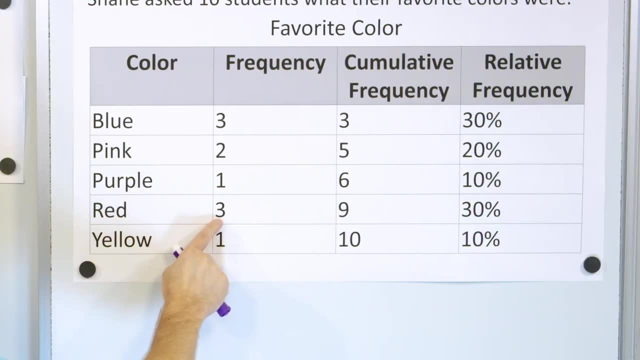 answered blue? How many people answered pink? We only have one here and one here, That's two. How many people answered purple? Only one person answered purple. How many people answered red? 1,, 2, 3 people answered red. 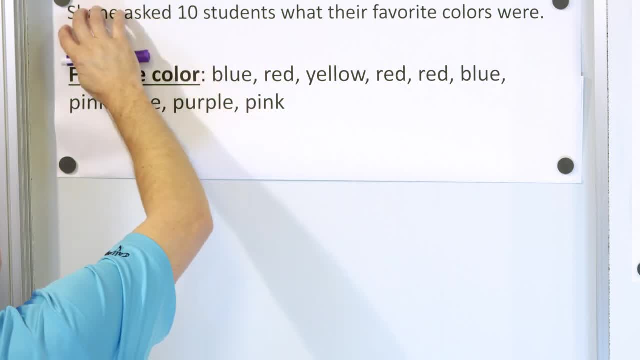 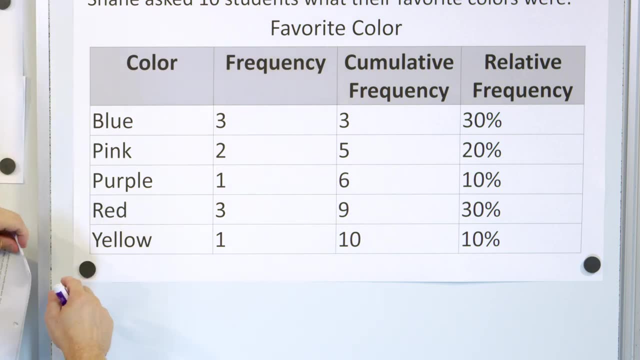 How many people answered yellow And only one person answered yellow. So, again, it's difficult to look at this and understand, But when you look at this it's very easy for you to see. okay, the people who picked purple and yellow were the least, most common, the lowest frequency. 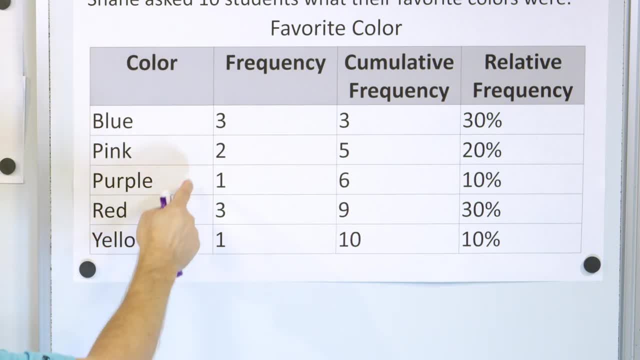 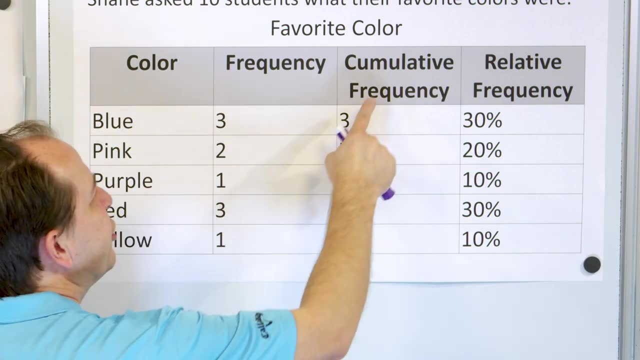 where it seems like people like red and blue the most, Followed in second place or, I guess, in third place. however, you rank it by pink, So it's easier to digest it from the table. Now, the cumulative frequency: the very last line item should always be the number of respondents. 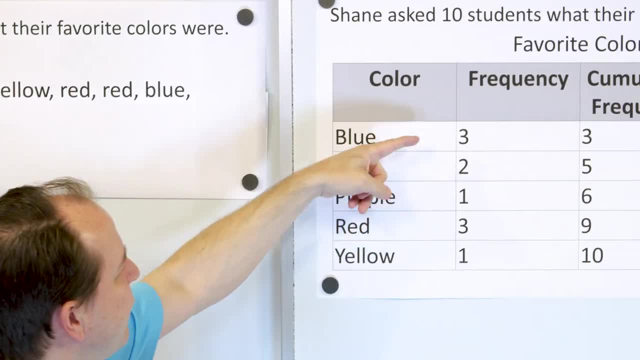 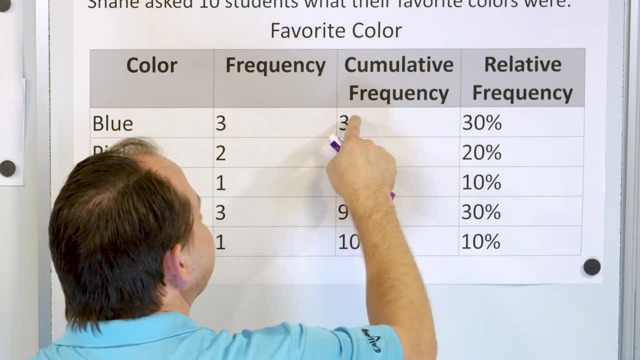 Notice that we asked 10 people. We have 10 answers here. So if we add these up, 3 plus 2 is 5, then 6, then 7,, 8,, 9, then 10.. There's 10.. The way we construct this is the first line in the 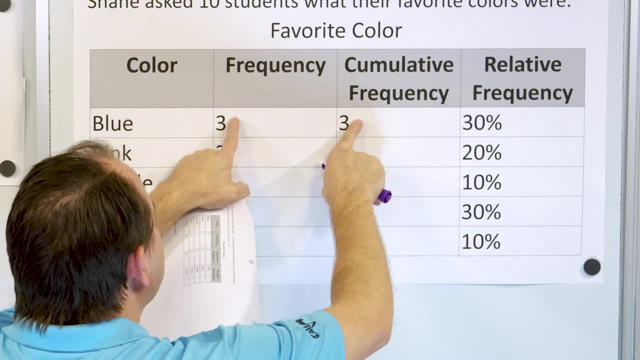 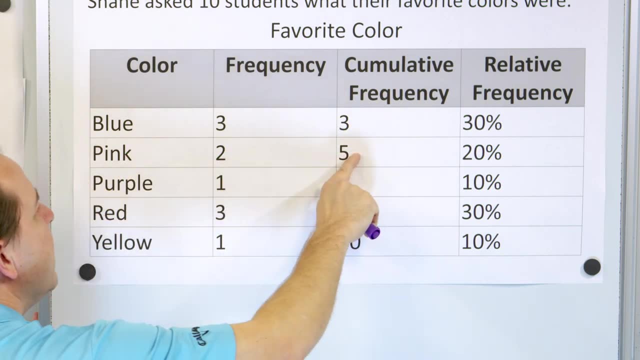 cumulative frequency is just this number And then, however many we get for the next one, we add them together and get 5.. So 5 is the new respondents here plus how many answered before. Then for this line it's the new respondents plus how many answered before to 6.. Here it's the new respondents. 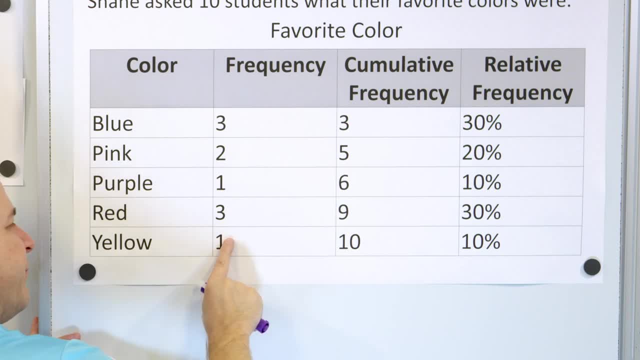 before. 6 plus 3 is 9.. And for here it's how many new respondents plus however many answered before, which is 10.. So the bottom number should always be the total amount of answers. you have the sum of this column, in other words. All right. Next we calculate the relative frequency. 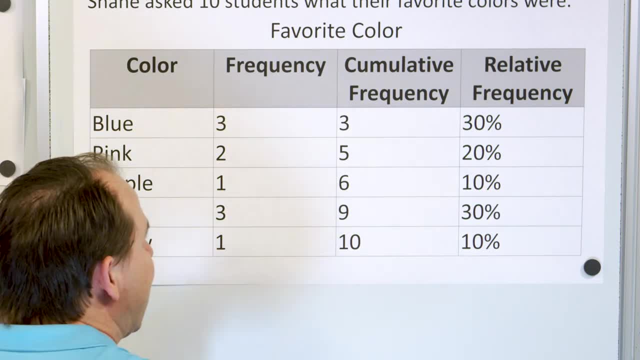 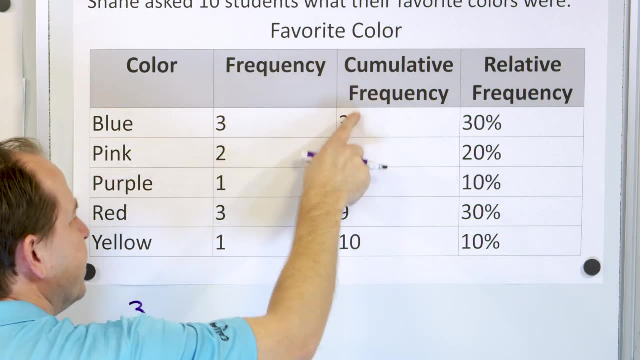 And these numbers work out to be really, really nice, because, if you look at it, what's the relative frequency of this one? It is 3 people answered out of a total of how many There's 10.. The cumulative frequency at the end is just 10 people, 3 out of 10.. Now, when you divide, 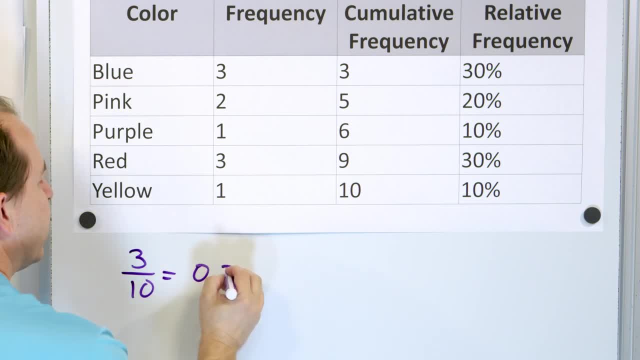 by 10, you just move the decimal one spot to the left: 0.3.. And then, as a percentage multiplied by 100, it's 30%, And so we have 30% here. For this one, it's 2 out of 10.. It's the same sort of thing. 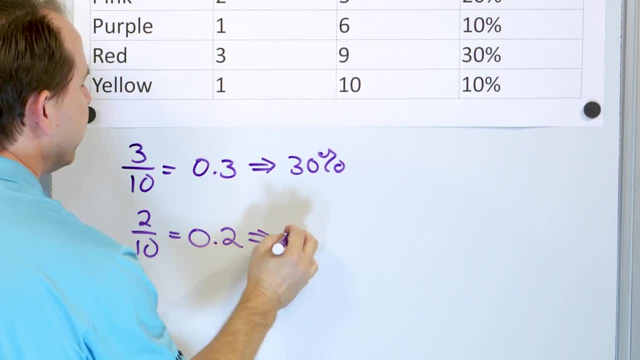 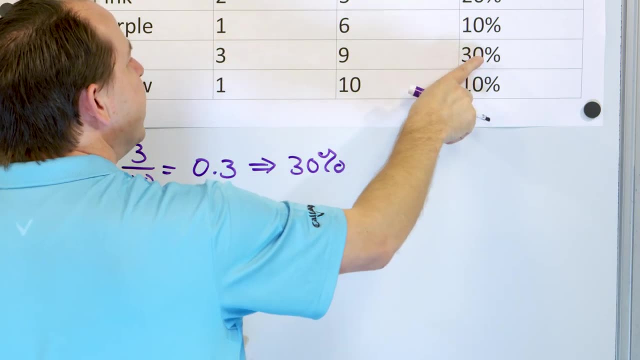 2 out of 10, 0.2,, which means 20%, because we moved the decimal two spots here. For this line, it's 1 out of 10,, which works out to 10%. For this one, it's 3 out of 10,, again 30%. For this one, it's. 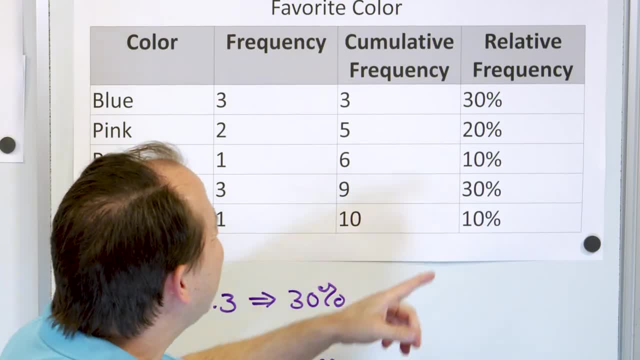 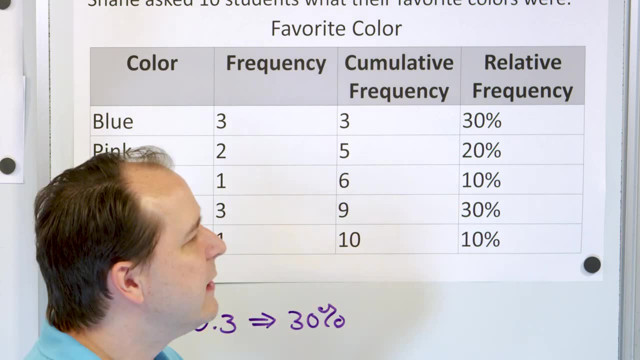 1 out of 10,, again 10%, And, as before, if we add up all the percentages, this becomes 50, then 60,, then 70,, 80,, 90,, then 100%. The relative frequency should add up to 100%. Now, this is nice because you can look. 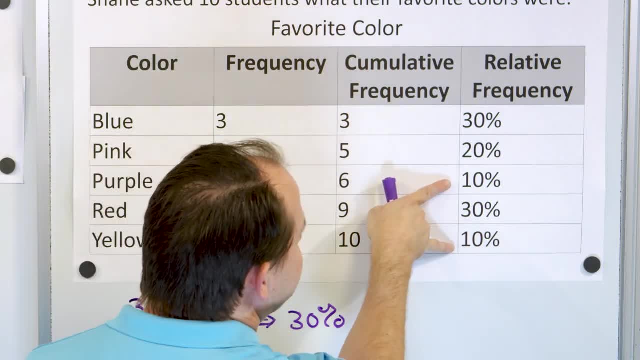 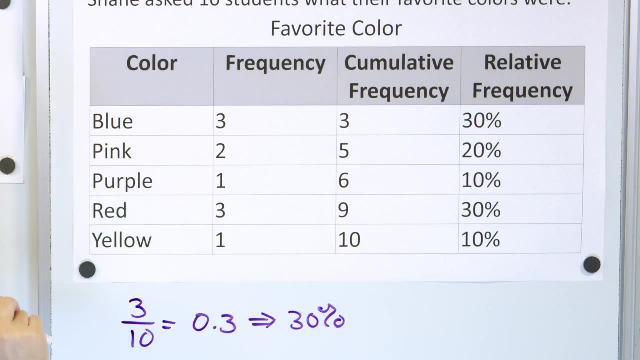 right away and say: okay. the least popular colors at 10% of pop is purple and yellow. The most popular colors, at 30% each, were red and blue, And that is a much better way to present this data in a frequency table with a cumulative- I'm sorry, a relative- frequency in a percentage. 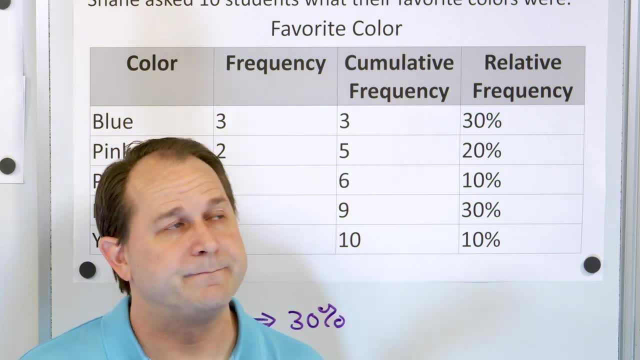 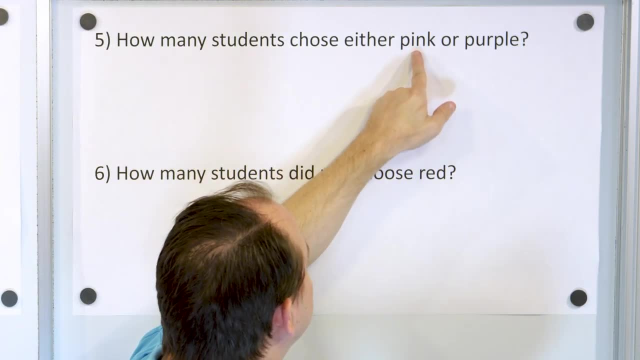 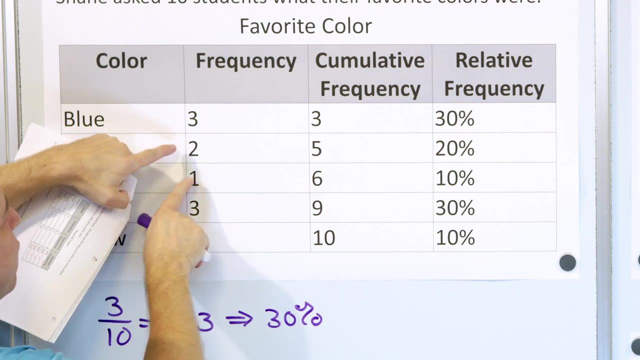 because then you can just easily digest what the data is telling you all. right Now let's take a look at our first actual problem. How many students chose either pink or purple, pink or purple. So we look in the pink, we look in the purple. How many students, how many respondents together? Two plus one is three. 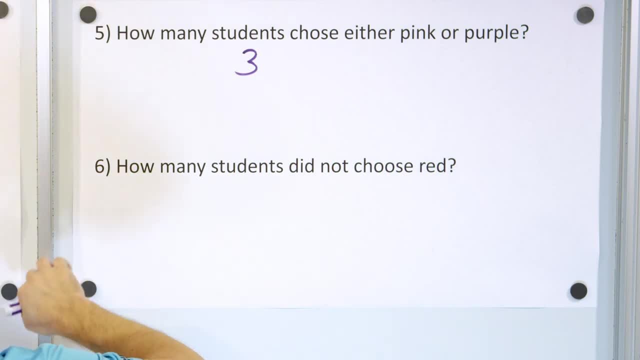 So only three people chose pink or purple. You can get this answer by going to the raw data and counting, but from the table it's much faster, especially if the data is very long. How many students did not did not choose red? So here's red. So how many people did not choose red? Well, that will be. 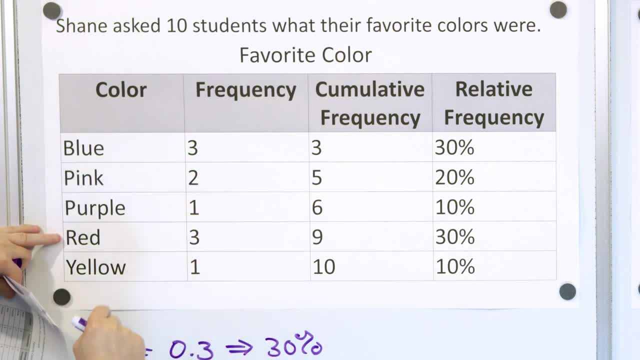 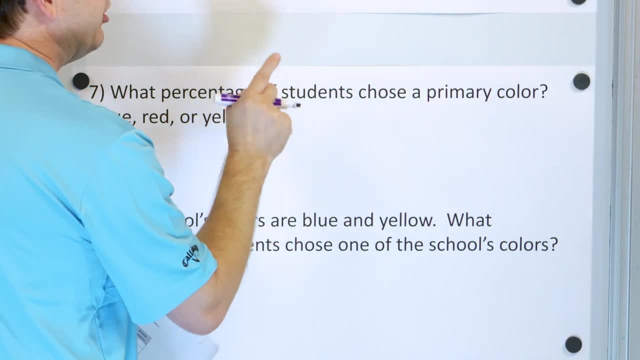 three plus two is five, then six, then seven. We skip over that for seven. How many people didn't choose red? Seven? Next problem: What percentage of students chose a primary color which is red, blue or yellow? What percentage of students chose a primary color- red, blue? 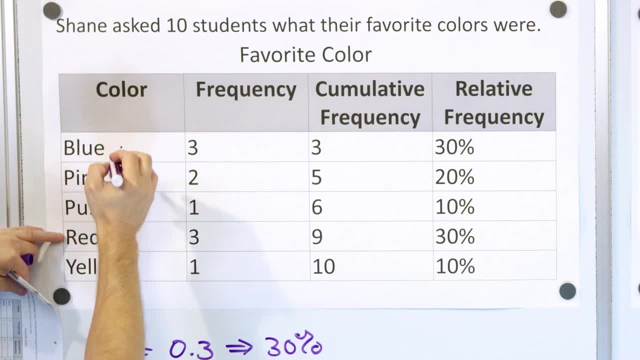 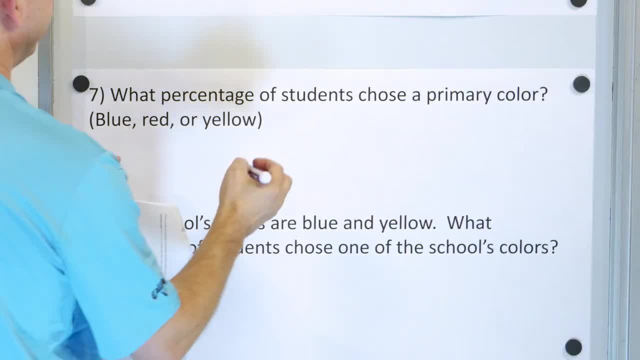 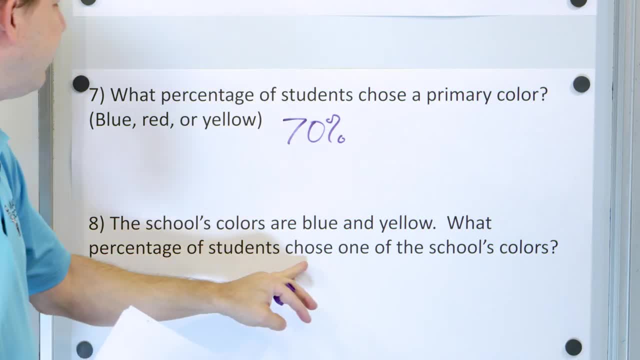 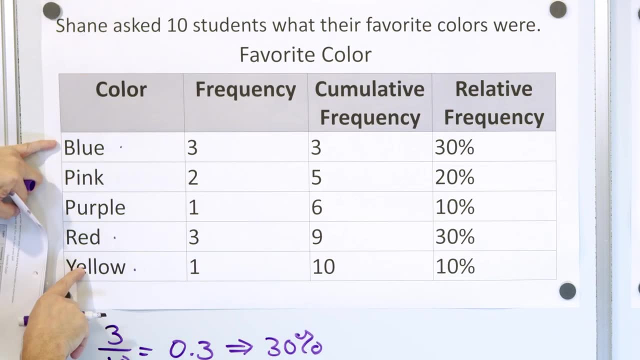 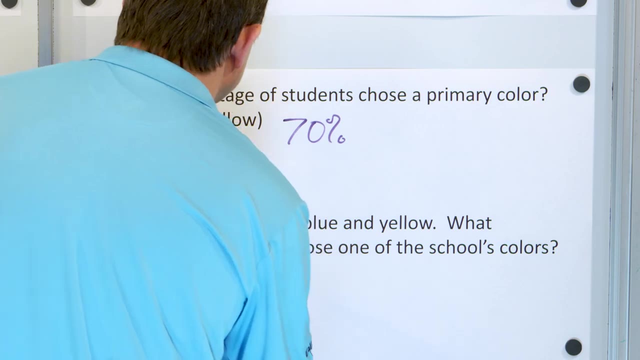 colors are blue and yellow. What percentage of students chose one of the school's colors, either blue or yellow, Right? So here is blue, Here is yellow. 30 plus 10 is 40. So 40% chose either one of those 40%. So this lesson hinged on kind of two things. Number one: